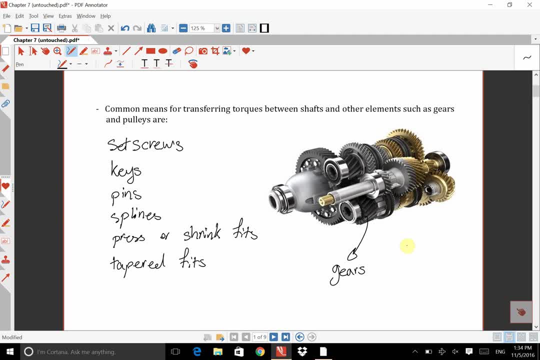 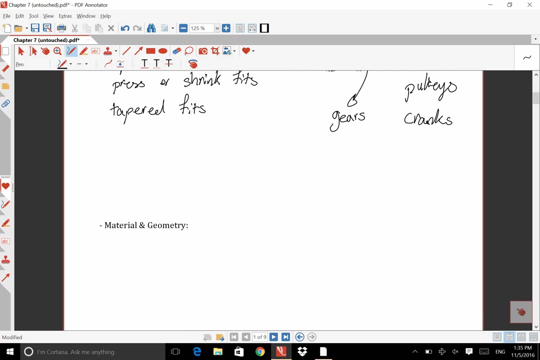 could have pulleys, for example. we could have cranks or any other things that like we can have, like sprockets or anything. i'm gonna, i'm gonna move and i'll let i leave it to you to read those parts by yourself. i'm i'm going to talk more about the problems that we're going to see in this chapter. 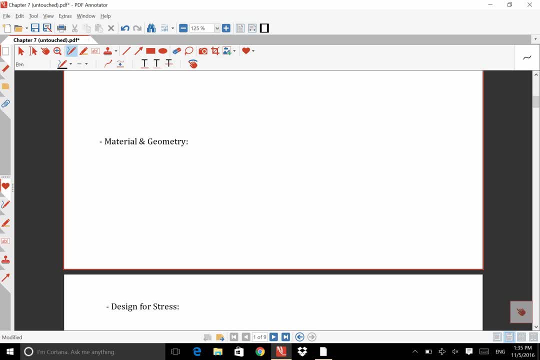 material and geometry. there's a term here. this is called rigidity. rigidity of a shaft or of any system is defined as modules of elasticity times I, which is second moment of inertia in shafts. usually shafts are made of steel and e modules of elasticity. 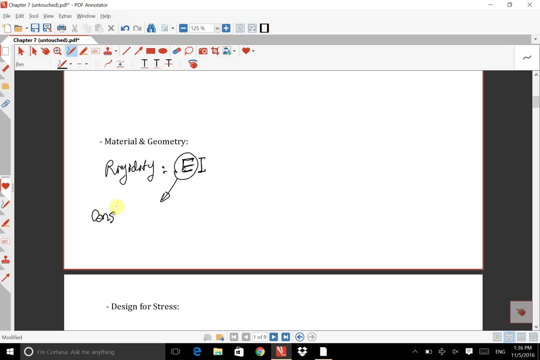 is almost constant of the for all steels. so if you want to control the rigidity- and this E doesn't play any role here, so this I can control the rigidity. and, as you said, if we have most of the shafts has a round circular, so if you have a circular cross-section, this I 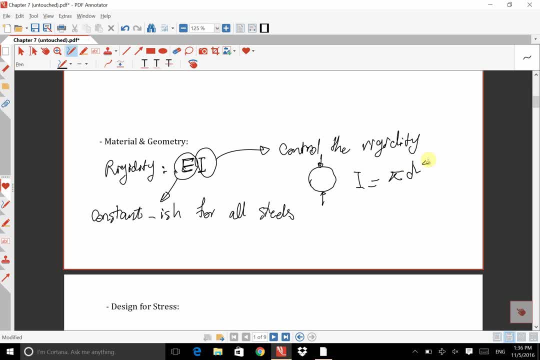 will be P, D to the power of four divided, but by 64, where D is the diameter. so if you want to control their rigidity, we need to play with the diameter here, and by playing with the diameter we can change the eye and we can extend to their rigidity. 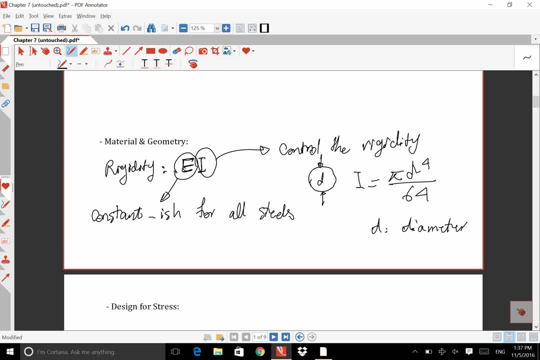 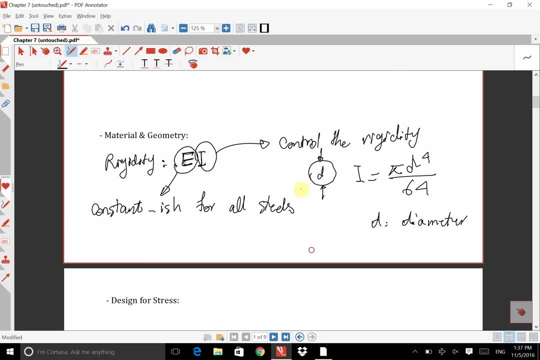 if we change the material, it really doesn't do any helps for us. when you want to change the rigidity of a system, okay, let's move on. design for stress: we can have different type of loading in any system loadings. we can have axial loadings. 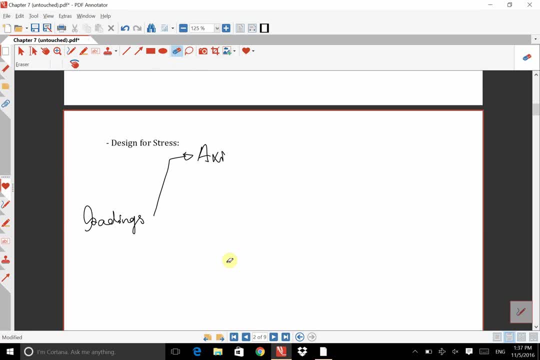 axial. so if i have an axial loading, the stress will be normal sigmas and the amount of stress will be the axial force divided by cross-section area. so if this is my shaft, if i have this force here, which is p, and this is my shaft, and if this is my area a, the amount of stress will be p over a. i can have bending loading. 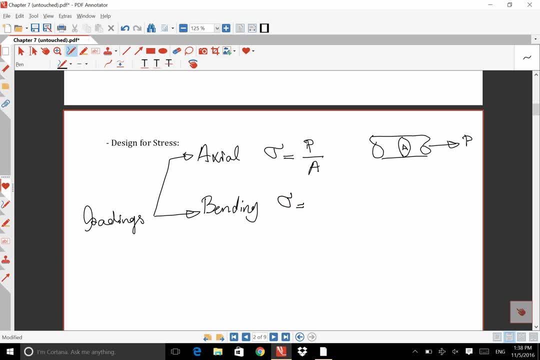 in this case, stress will be again normal and the amount of stress will be m rho over i, and rho is a distance of the point that we are analyzing from the descent of the center of the cross section, but here, because we are looking at the critical points, 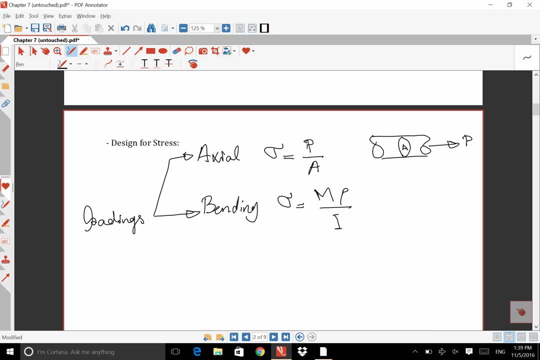 so we are looking at the maximum stresses, and the maximum stress happens when rho is in its maximum value and maximum row happens when rho is equals to r. so, for example, if i have the same shaft under bending moment, i can see that my Texas and my c star is holding the same distance. 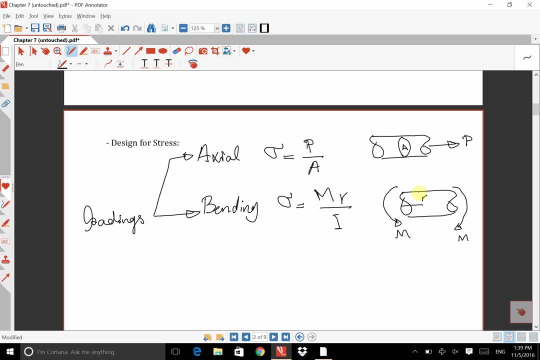 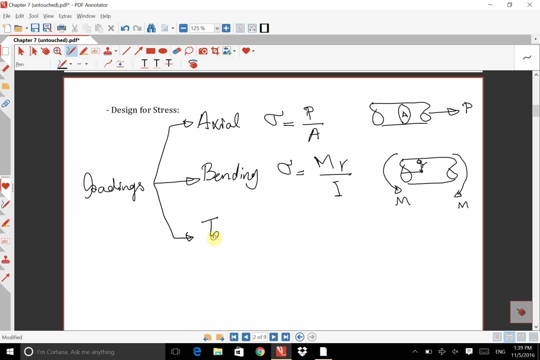 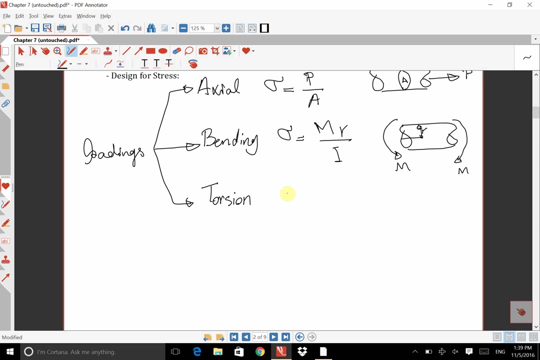 and if this distance is r the radius, the maximum stress is mr over i. another type of loading that we might have in a system is torsion. torsion makes a stress, but this time this stress is not normal. so because we can have thicknessing of the seizure skew when stress is not normal, so this radius of the glossyð is Add spicy. so we're not exaggerating about this and musing. the pressure Ying is equal to at leastoliola in this system. doesn't matter, just that, just under 911 mN. then you have the present stress in coolug. 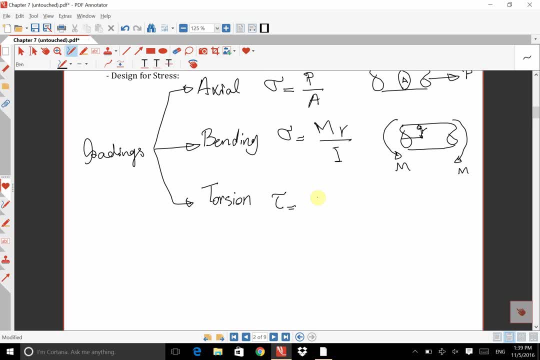 and that will be a shear stress. and the amount of that shear stress will be T? rho over J, and J is the second polar inertia of the shaft- and the maximum shear stress will be when rho is equals to its maximum value, which is R. so if I 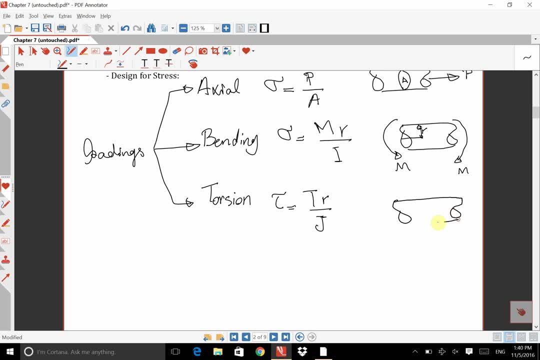 have shaft like this and if I have a torque like that, the shear stress will be T? R over J. okay, for example, for the first part, when you have normal stress, then it's P over A because the cross section is a circle, so the area will be B P, R to the power of 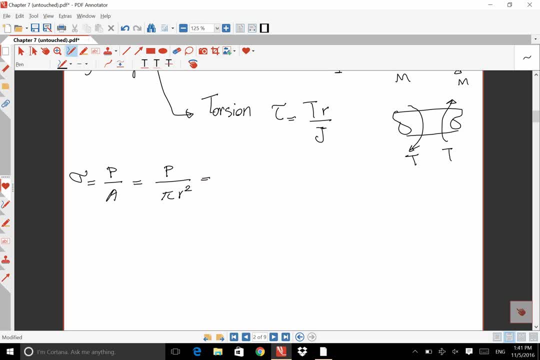 2. so if I want to change this one, I'll write it based on the geometry, that will be 4P over PD squared. ok so, and this is happens when we have axial loading, so i wrote the stress based on the diameter and the amount of force: axial force. 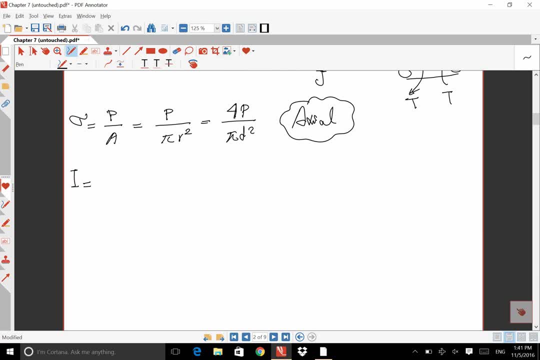 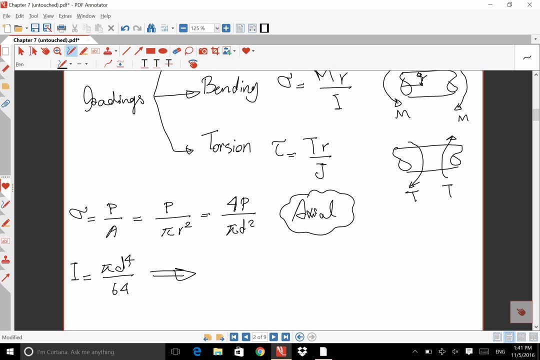 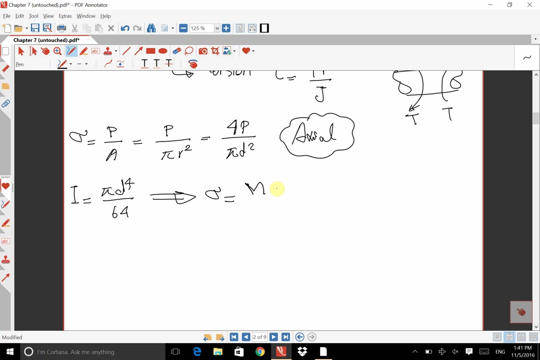 second moment of inertia for a round cross section is p d 4 over 64. so if i substitute that one into this equation here, the amount of normal stress for bending loading will be m r, which is d over 2. and here i'm gonna write this i, which is p d to the power of 4 divided by 64. 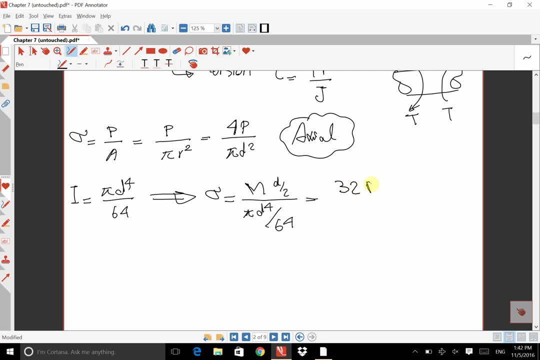 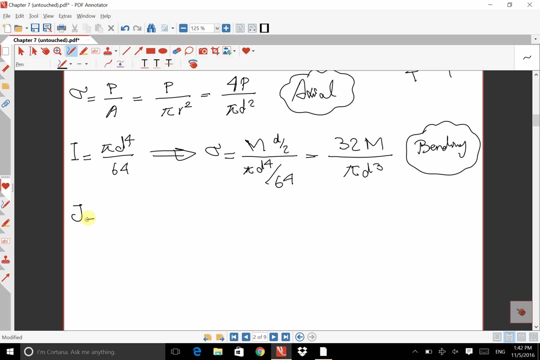 so at the end of the day i'm gonna have 32 times m divided by p? d3, and this is when i have bending loading j second polar inertia is p d square d to the power of 4 over 32. and if i substitute that one, 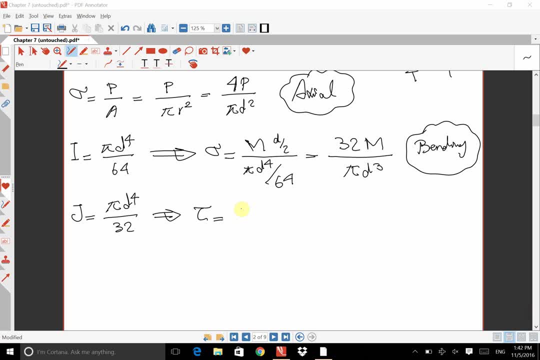 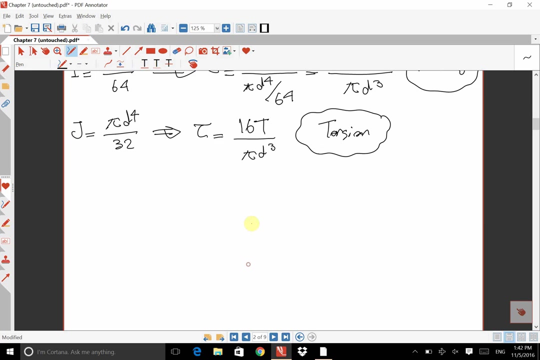 for the torsion stress, i'm gonna have 16 t p d cube after simplification, okay. so these are the stresses that for each loading. uh, okay, what i'm gonna do here, i'm gonna write, i'm gonna look at a very arbitrary situation. for example, 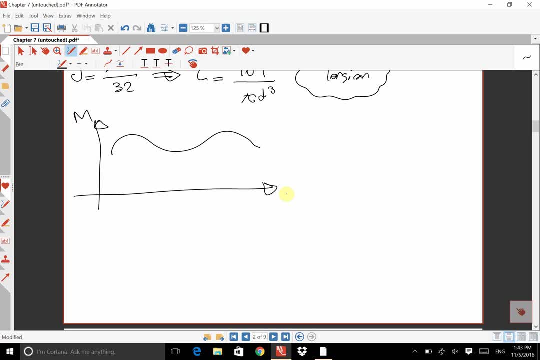 if this is my moment, the behavior of moment with respect to time, if i have a general fluctuation like this, this general fluctuation, for example, it has an offset of something. so if this is m, this offset, i call this one m, m, m of m, and i call the amplitude. 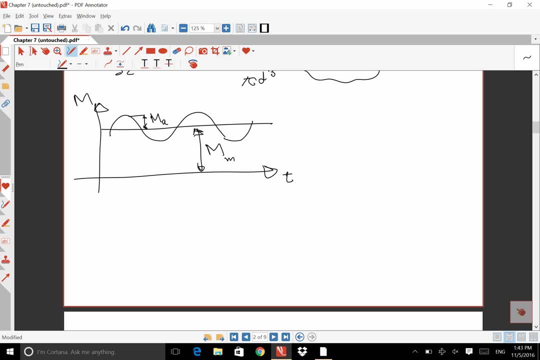 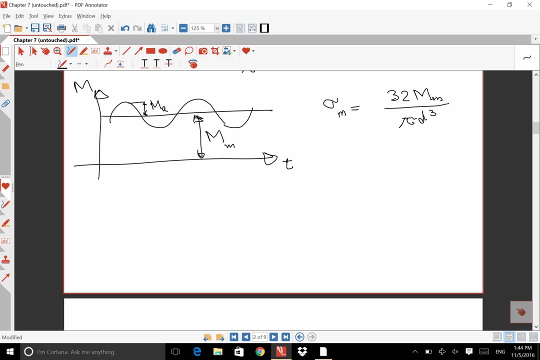 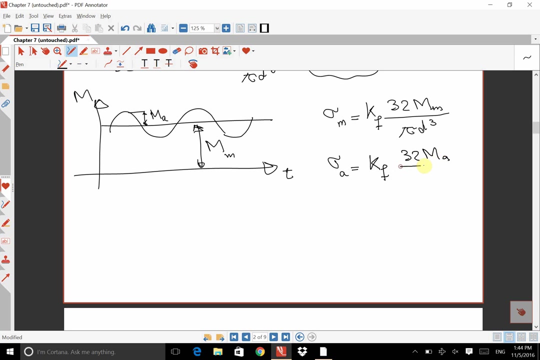 m a. okay, so i can say the sigma m m is the. I'm going to have fatigue stress concentration here, So that will be my sigma m. And the same thing is valid for sigma a, which is kf32ma over pd. cubed In these two equations, mm is the offset. 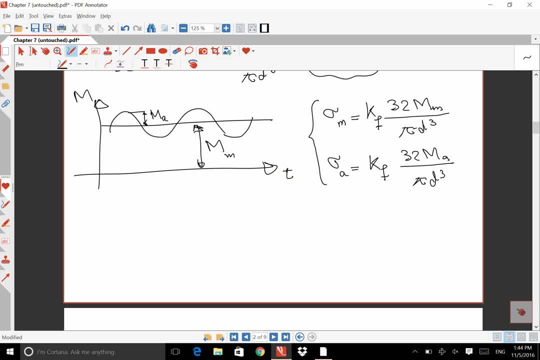 of oscillation from the time axis, and ma is the amplitude of oscillation. Okay, If this graph was for torque, this value could be tm and this could be ta. So it doesn't matter what I'm looking at. if it's a general case, if this is moment, this is mm. ma. If this is torque, this is ta, tm. If 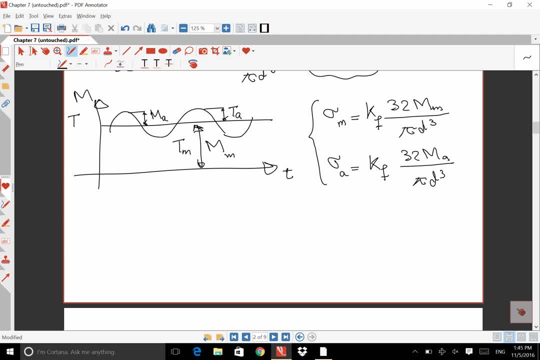 this is a stress, this is sigma m, sigma a, if that's normal stress. So I can say: tau m, which is shear stress, equals kf16 tm over pd pd cubed, and tau a, which is kf16 ta over pd cubed. Okay, If you have any questions about these, 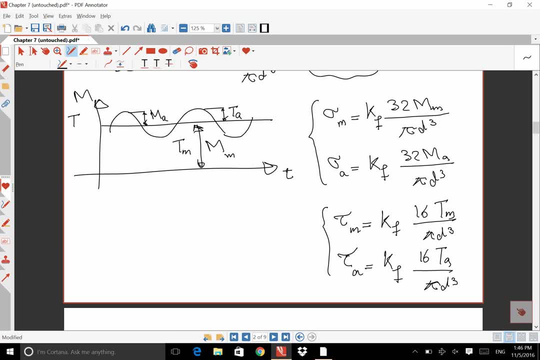 things. you can restudy chapter six. Okay, In this chapter usually axial loading doesn't make any differences And usually we neglect the axial loading. So when we are designing a shape, we're going to have to make sure that we have the right angle. 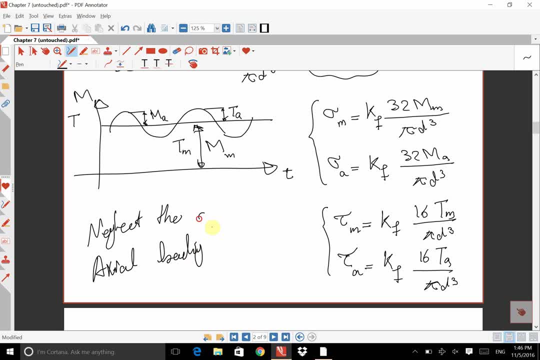 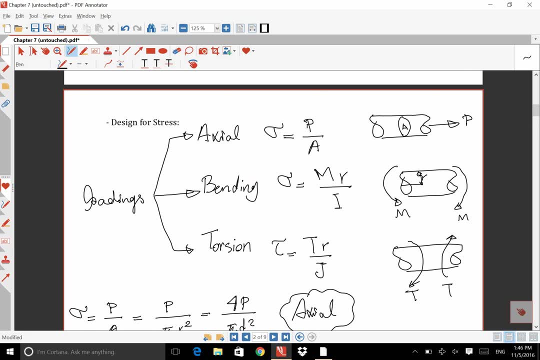 So we're going to have to make sure that we have the right angle. So we're going to have to make sure that we have the right angle. So when we are designing a shaft, the important loadings for us are bending and torsion, And usually axial loading are very small, so they can be neglected easily. 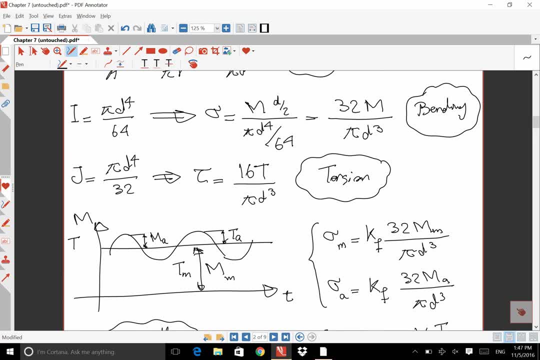 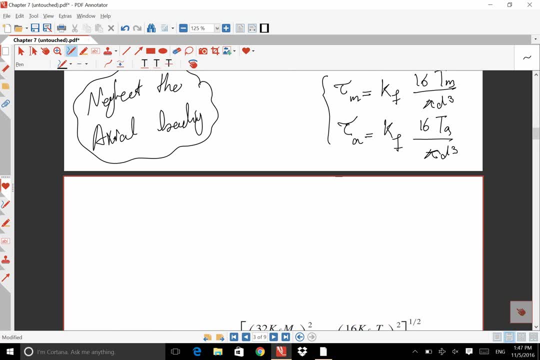 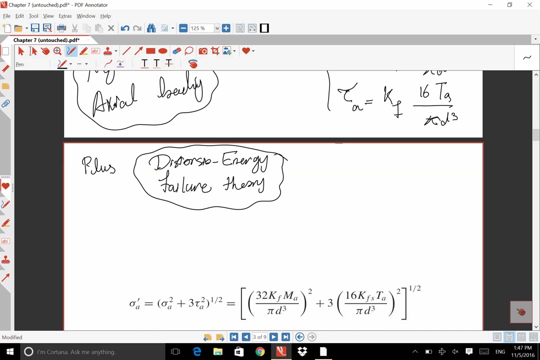 And it doesn't make any differences at the end of the day. Okay, So, after defining these stresses, these ones, we're going to have to address them. Those stresses, plus distortion, energy failure theory, like this one, will lead us to these two set of equations. 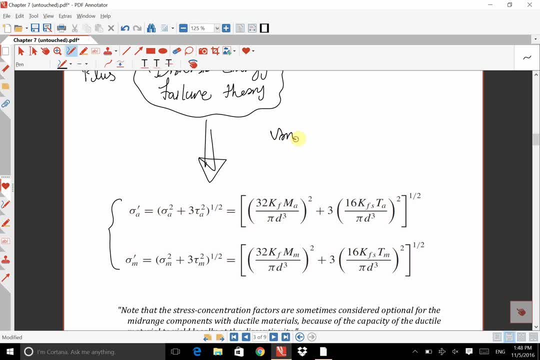 and these are von Mises stresses for rotating shaft. so that's important and the shaft should be solid and we neglected the axial loading. so we're gonna have Sigma, a prime which can be found from this equation, and we have Sigma, a previous sigma M prime, which can be found from this closed-form equation here, okay, in. 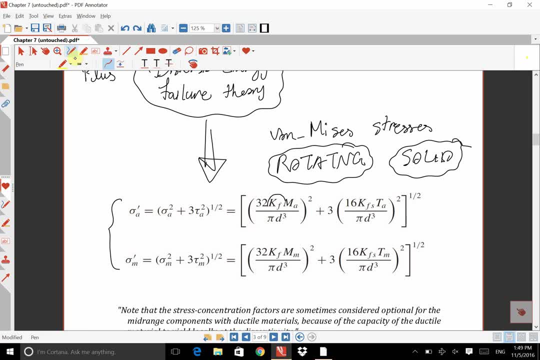 this. in this equation, there are a couple of factors that I'm going to talk about. one of the factors that is not that unfamiliar for us is KF. KF is fatigue stress concentration factor. I'm going to say fatigue factor, fatigue stress concentration factor. in chapter 6 we talked about KF and we talked about how. 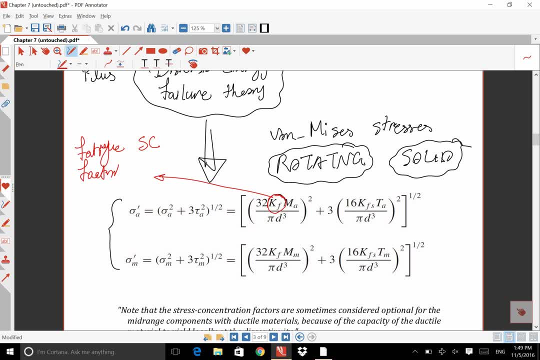 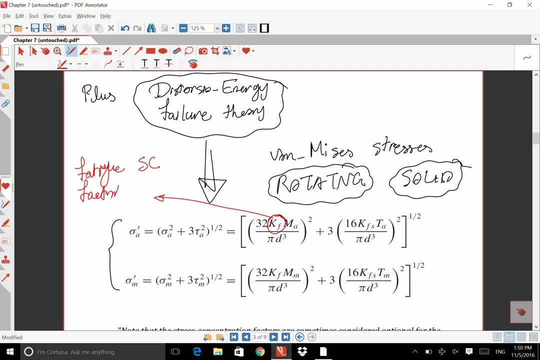 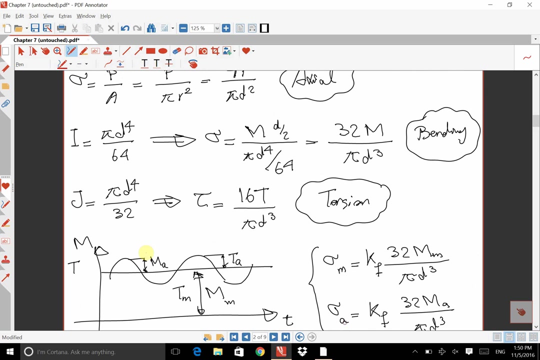 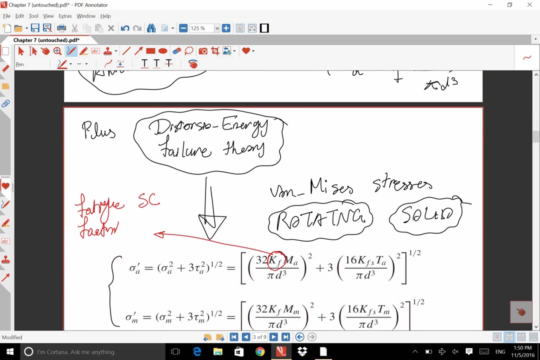 we can find KF from KT- theoretical stress concentration- and Q not sensitivity. KFS is fatigue stress concentration factor for shear stress. MA is the amplitude of moment which we showed in this diagram. this is MA, MM is the offset and TA and TM are amplitude and the offset respectively. there is one. 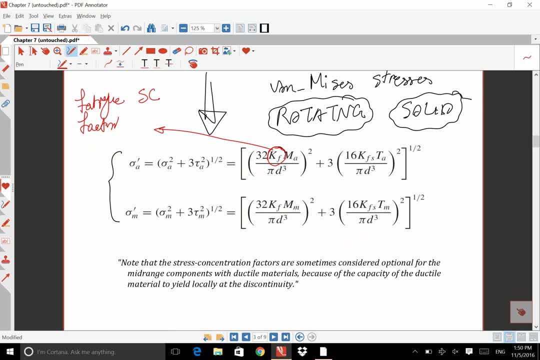 note here from the Shigley's book that I brought you at this point, and what it says is: note that the stress concentration factors are sometimes are considered optional for the mid-range components with ductile materials because, because of the capacity of the ductile material to yield locally at the discontinuity, 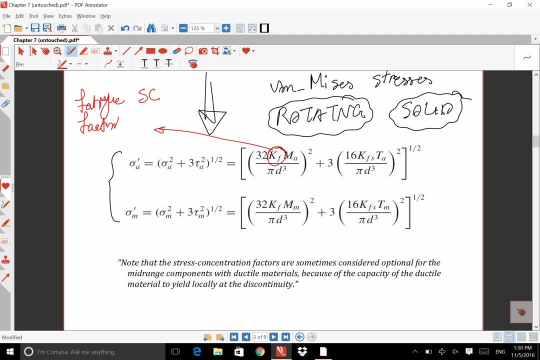 it means that sometimes we can, when we have a ductile material for mid-range components, for mm and tm, sometimes we can neglect this kf and kfs and we can assume that those are one. but if you want, you can use the tables and i do suggest you. 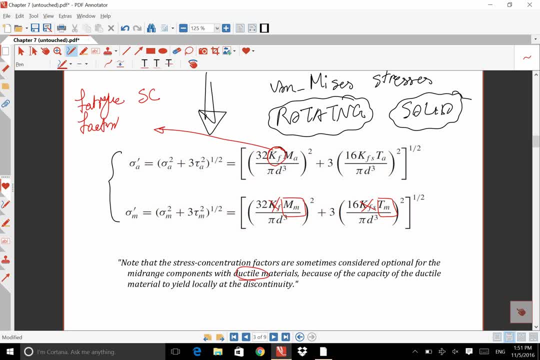 to use the tables and find the accurate value, especially when you are working for your final exam. but if you are, you can use the tables and i do suggest you to use the tables and find the accurate value. working for a company and you just want to estimate a number you can just easily forget. 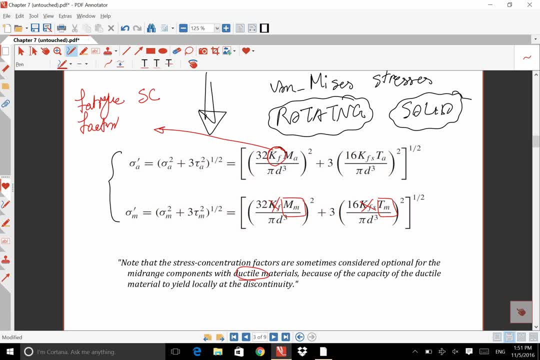 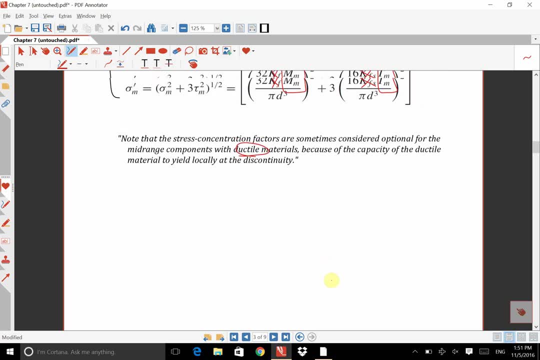 about that and just estimate some numbers based on considering those values. one: okay, when we are talking about designing a shaft- if that's our shaft- and usually we are talking about suggesting a diameter for the shaft- sometimes this diameter is very important in order to have an accurate design. this diameter can be more than enough to make the shaft correct. but you also have to understand that the largest diameter of the shaft is pretty small, so that it is very difficult to adjust the length of the shaft, and so you always need to figure out how to adjust the length of the shaft when you are designing a good shaft. 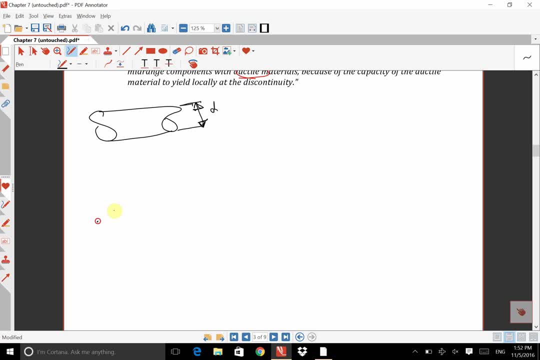 is known for us. so we could have two type of question. in one type of question d, diameter is unknown and is asked, and in the other type of question, d is known, if diameter is known for us, and we are asked to find the factor of safety. what we can do is we can just do the method that we learned in chapter six. 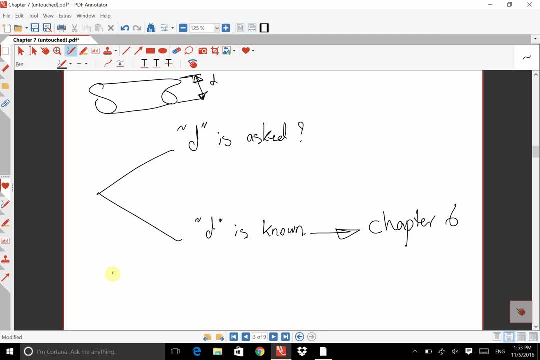 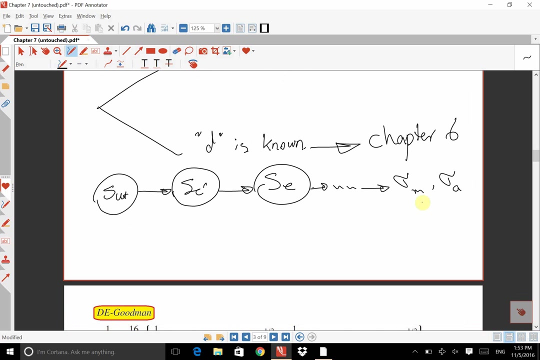 and we can find s u t s a prime. this is what what we talked about the other lecture s e and stress concentration factors and at the end of the day we can find sigma m and sigma a for one type loading and we, if we have a combined loading, we can find sigma m prime and sigma a prime, and then we can go to. 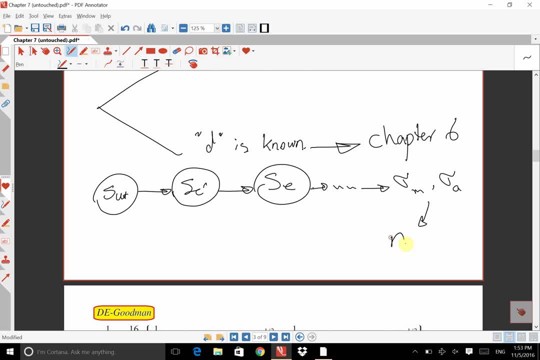 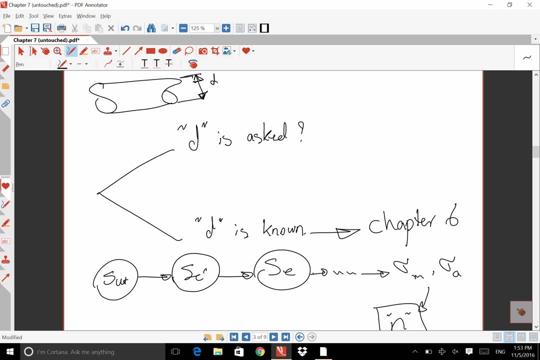 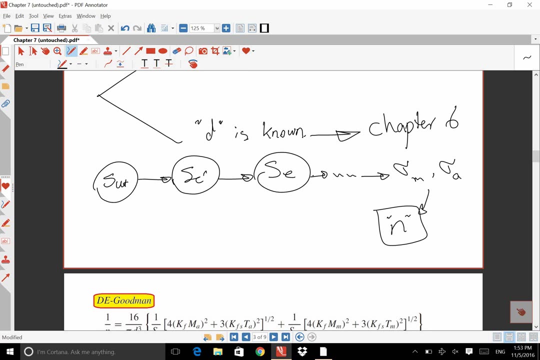 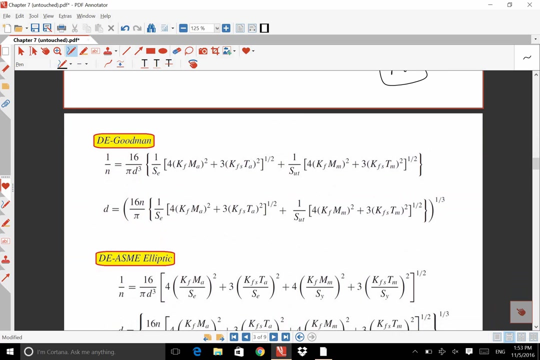 a closed form equations and we can find n safety factor based on some closed form equation. sometimes, when we don't know about d. we cannot use these type of, we cannot use this process because we don't know what d is in those questions. what we need to do, we need to use these kind of equations. 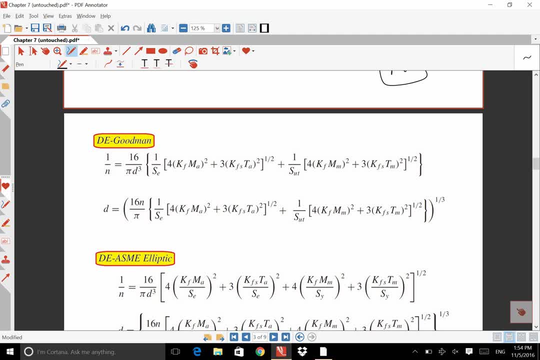 i copied these equations directly from the book. so for the first one, which is d e, goodman, this d e stands for and this store gen energy. okay, this storage and energy failure, it has a combination of goodman criteria and distortion energy failure. so for each, for each, criteria. here we have two equations, one of them. 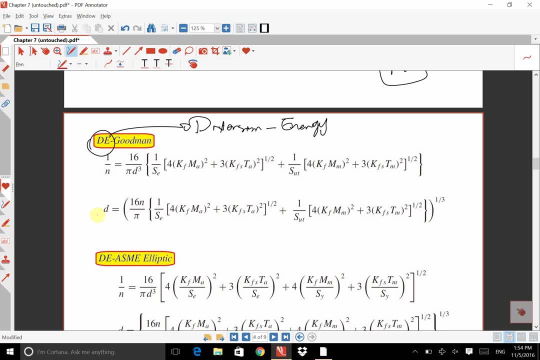 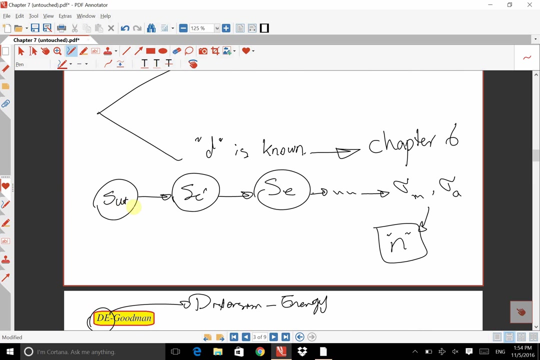 is based on d, so we can find the diameter, and in the other one we can find the factor of safety. so if you are asked to find the factor of safety based on distortion, based on Goodman criteria, you can use either this equation or you can come back and do what we learned in chapter 6 and we're gonna have the same thing for. 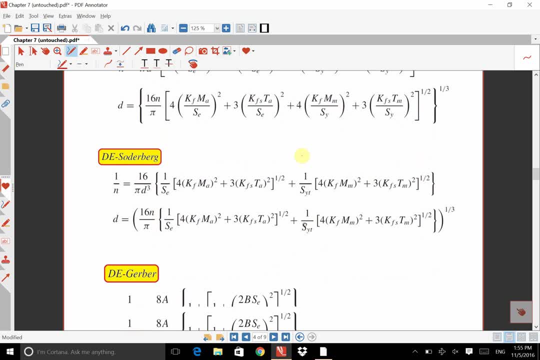 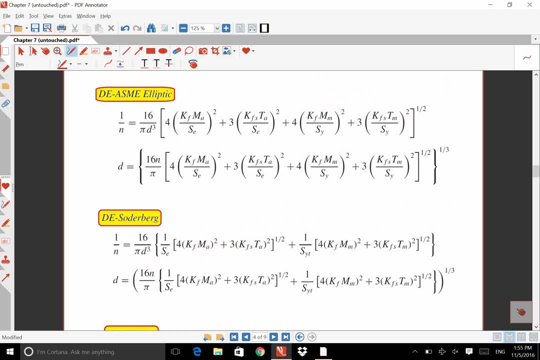 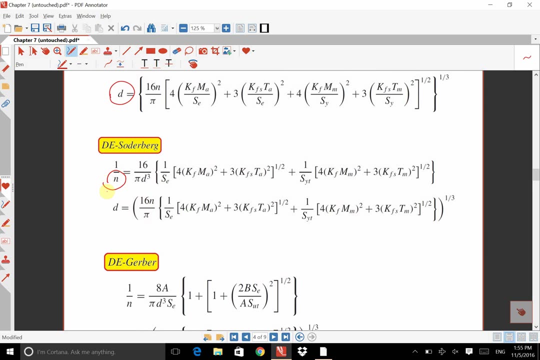 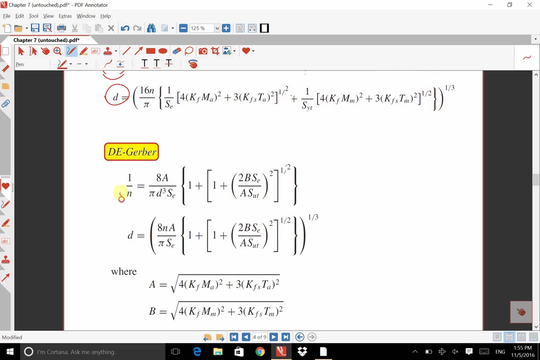 ASME, elliptic criteria, Soderbergh criteria, Gerber criteria. so for each criteria we have two equations: one of them is for finding safety factor, the other one is for finding diameter and D for Gerber. again you have the same things. you have two equations, one for N, the other one for D. 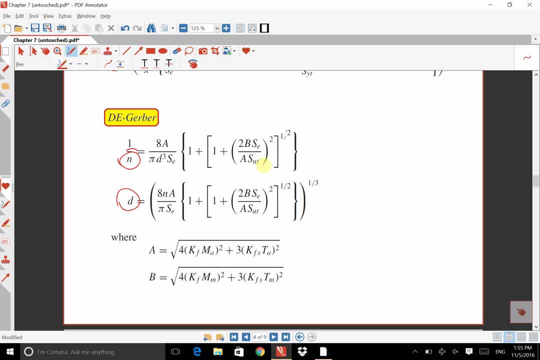 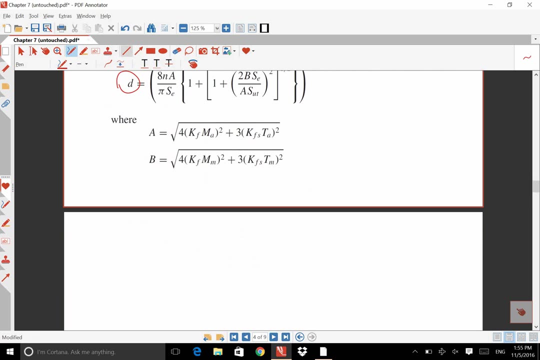 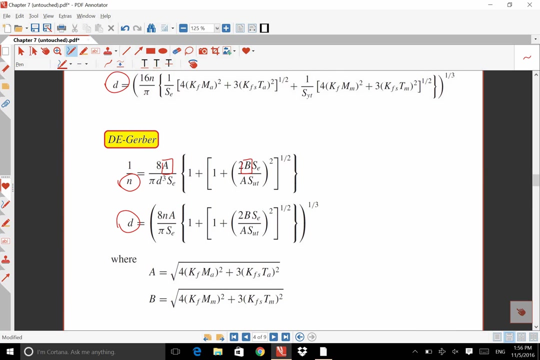 and because we wanted to write it in a simpler way, we have two parameters here, A and B, which can be found from these two equations here. okay, before I want to continue, I want to mention something at this point. sometimes we have steady torsion or a steady moment, for example. I'm going to 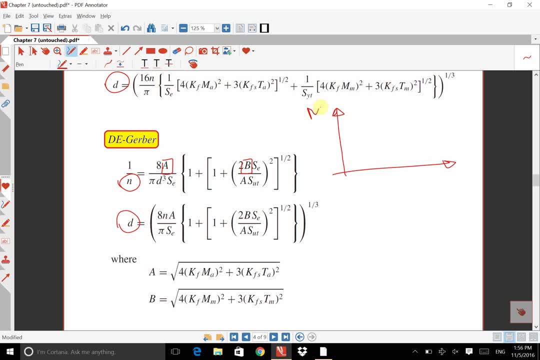 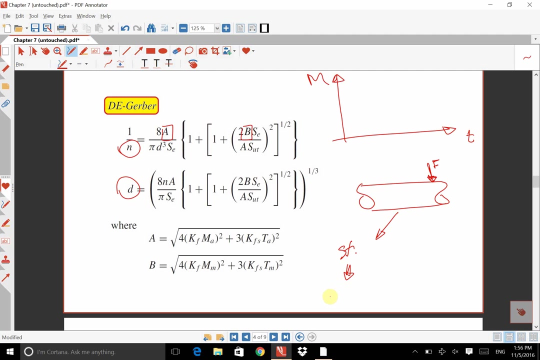 study two cases: if that's M T diagram for this shaft, if I have a bending moment, or if I have a force, like some forces, that makes bending in the system on this shaft, if this shaft is not rotating, if this is a stationary, the system will be static. so what we face here is what we learned in solids. 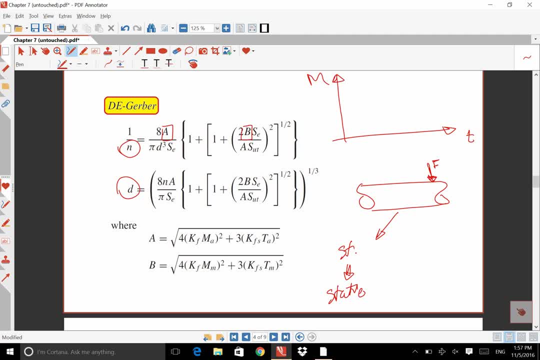 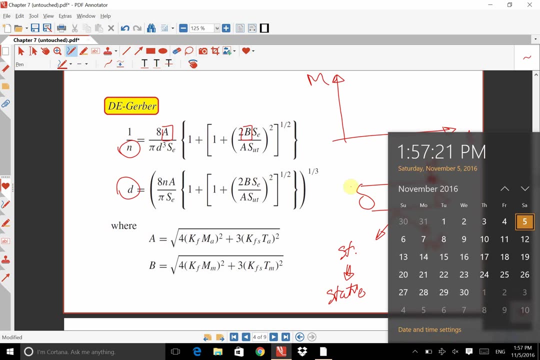 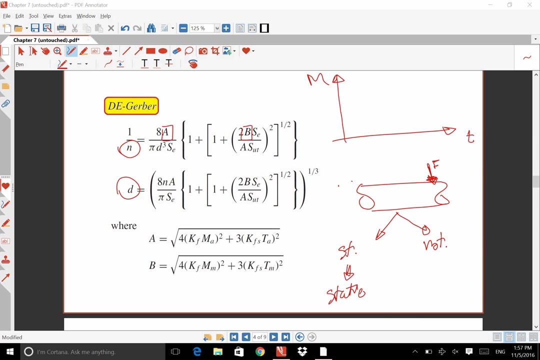 one. so that's a static type of loading and a system. so there is no fatigue here because we don't have any cyclic load on that. but if this shaft is rotating under the same amount of force, we're gonna face a cyclic load and in this case our fluctuation will be completely reversed. 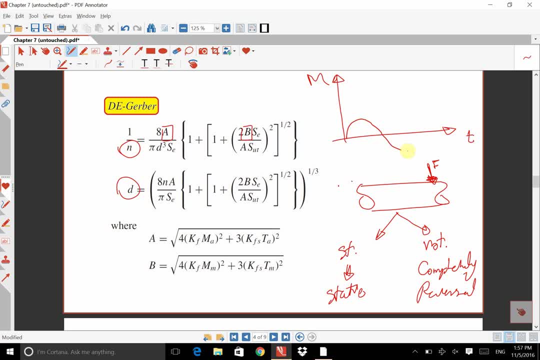 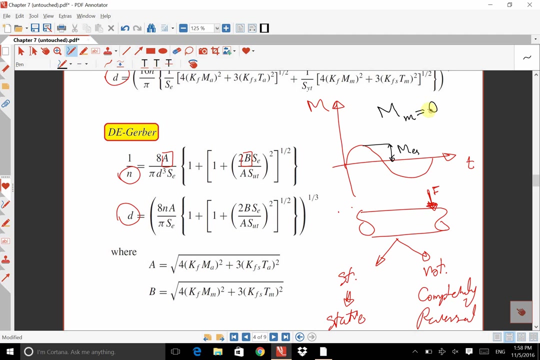 so we're gonna have this case here. so if that's the case, this will be m8 amplitude, but the offset in this question is zero. so mid-range M is zero because in completely reverse scenario we are a starting from zero, we are going to maximum tension and then we go to maximum compression. 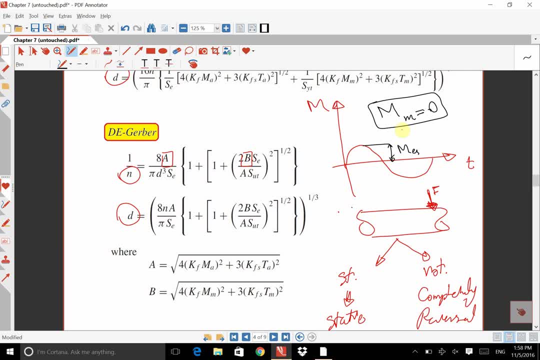 this is a definition of completely reverse scenario. so in such a case mid-range a moment is zero. so if we want to use any of those equations, we can just easily. for example, if I want to use a Gerber when I want to find B here I can just neglect this part because M of M is zero. 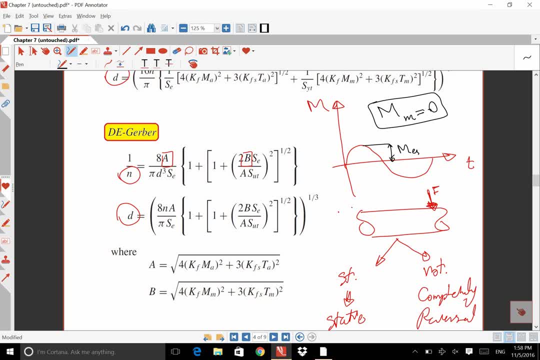 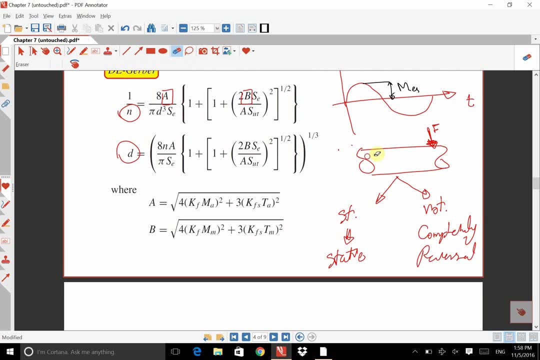 and it could be simplified to the square root of three times this guy here. sometimes I have. I don't have a fluctuation in the system. for example, I have a static torque like this on the system. this torque is not fluctuating. in this system i have some offset, which is tm, and because there 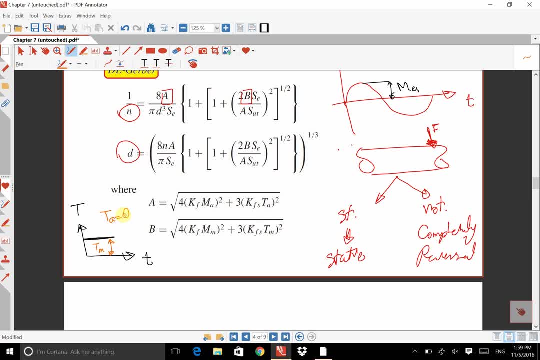 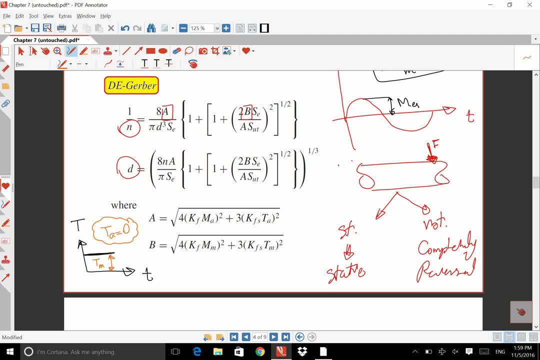 is no oscillation. ta the amplitude is zero. so again, if i want to, for example, use gerber criteria at this point, whenever i want to use a, i can just put ta equals to zero and i'm gonna just have two times kf times, ma okay. so whenever we don't have any oscillation, 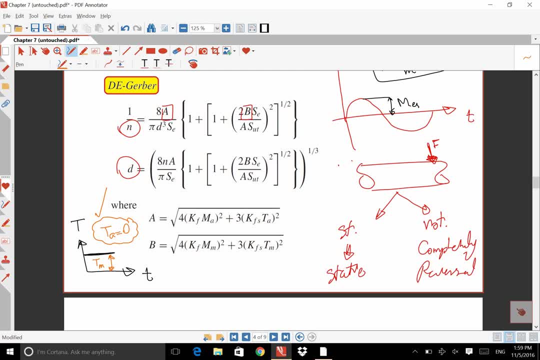 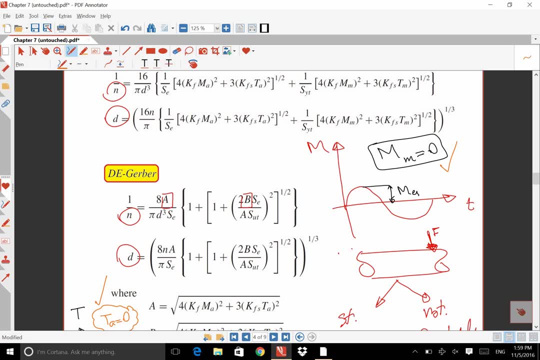 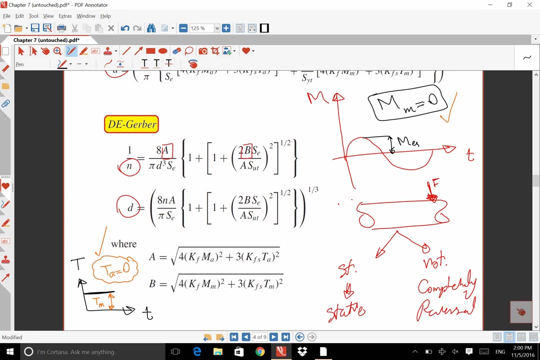 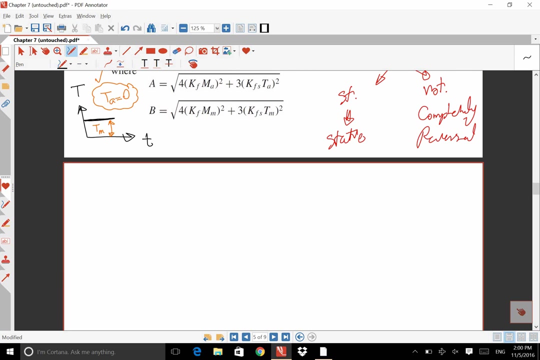 that means that the amplitude is zero. and whenever we have a completely reverse scenario, like, for example, in this example, that means the mid-range, m, or if that's for torque, mid-range, torque or mid-range, whatever it is, is zero. okay, um, static failure. static failure needs to be checked for all those scenarios. for example, 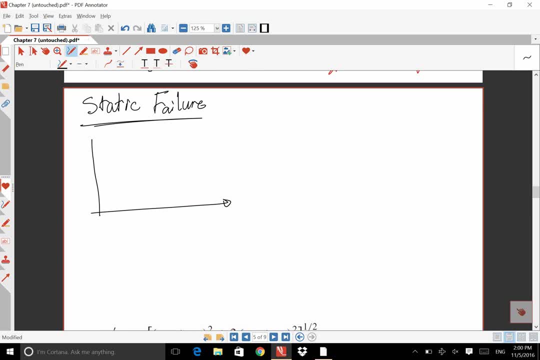 static failure has a number in it. so if we want to check for static failure, we just use static failure as the name of the scenario and that's it for now. if I have force time diagram like that, for example, if that's my static behavior, it means that, for example, if I, if I say my failure point is my yield point, this: 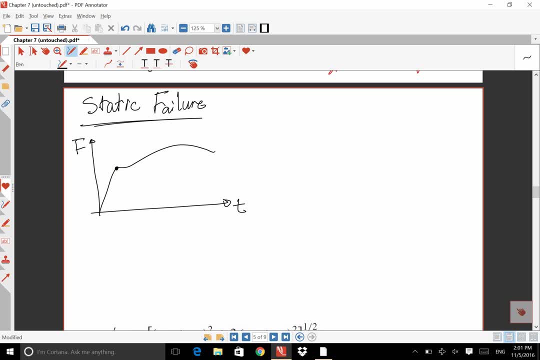 point for my purpose, for more for that specific purpose. so I cannot have more than this amount of load or the system will be failed. so in cyclic load we said that we can have a cyclic load and after a couple of cycles the failure could happen. and the amount of force that we needed, the amount of force that this is, 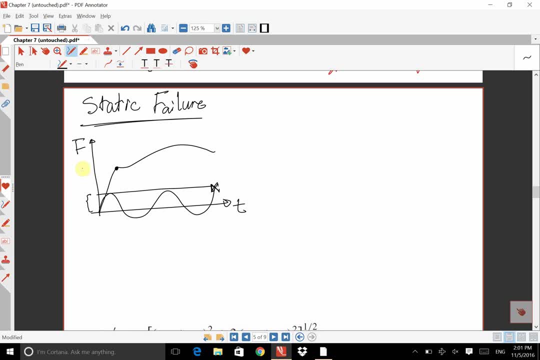 that this is needed to be failed is less than the amount of force in static failure and that was the basic of chapter 6. so we cannot have a fluctuation like this, because in the first cycle we're gonna pass this amount of load, the necessary load for static failure. so 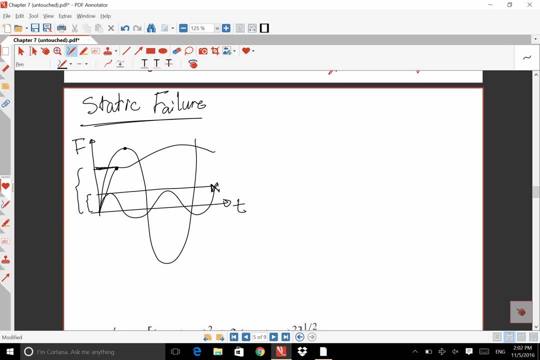 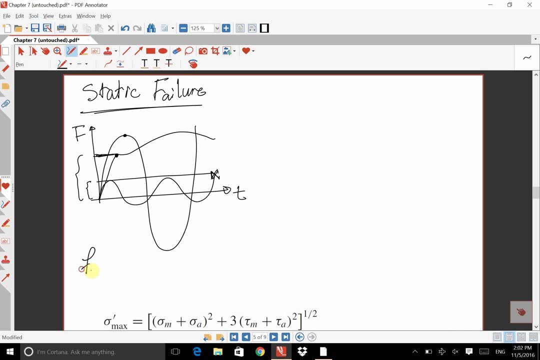 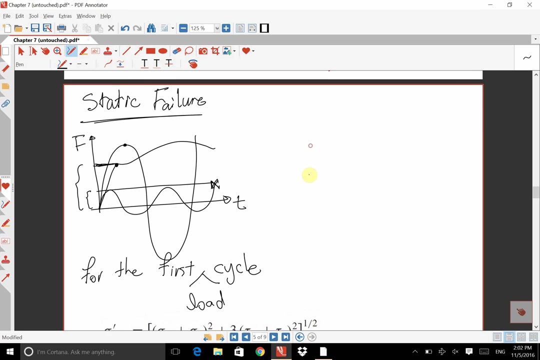 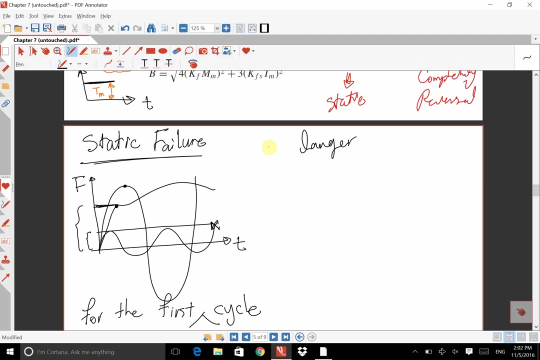 this is not valid for us. so for any of those criteria we need to check the static failure for the first load, I'd say for the first cycle, for the first load cycle. okay, Prim非常的, por favor. for the longer criteria, static failure will be checked automatically inside. 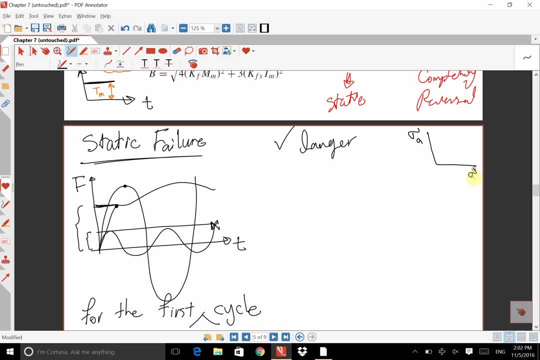 criteria is: remember the graph from chapter 6 where we plotted Sigma a versus Sigma m and we had couple of criteria here. you said that when we talk was covered. so when you want to use langer, you're not worried about to check the static failure, and the same thing is for soderbergh. 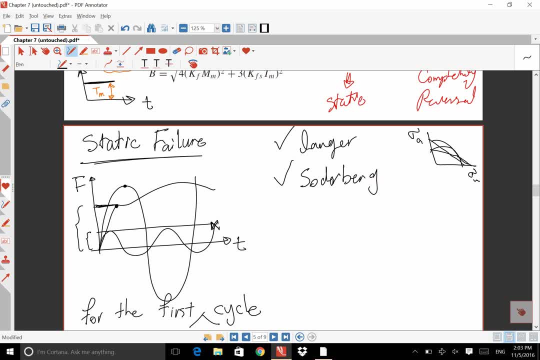 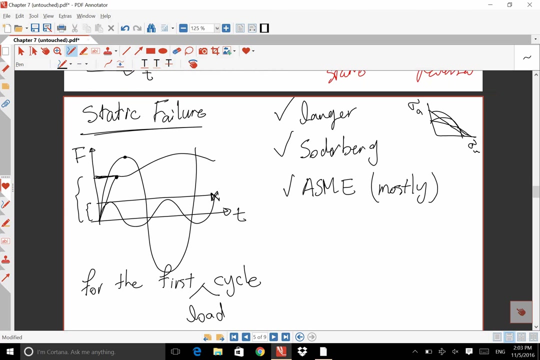 these are very conservative so you're not worried about that. about the asme criteria, mostly static failure is covered by this one. for the most of the graph it's covered, so maybe for 90 percent the static failure is covered in the criteria. but when we are using gerber, 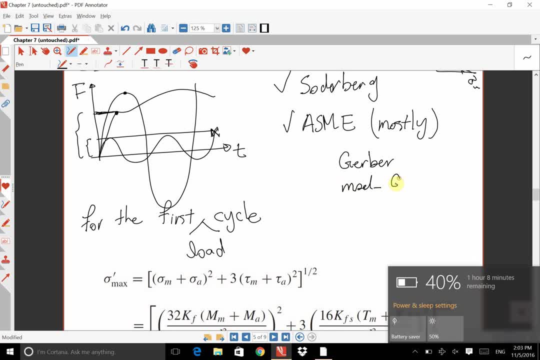 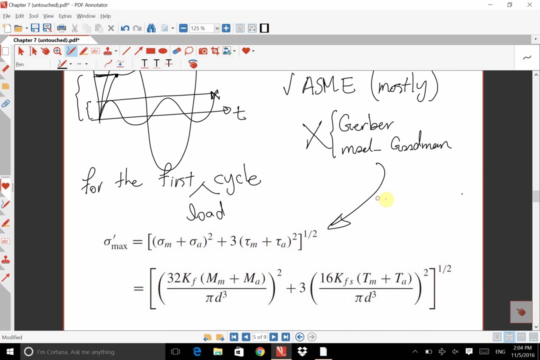 or when we are using modified and goodman criteria. for these two static failure is not checked inside the inside the criteria, so we have to check the static failure manually. in order to find a static failure for these two criteria, we need to define a phone mysys. 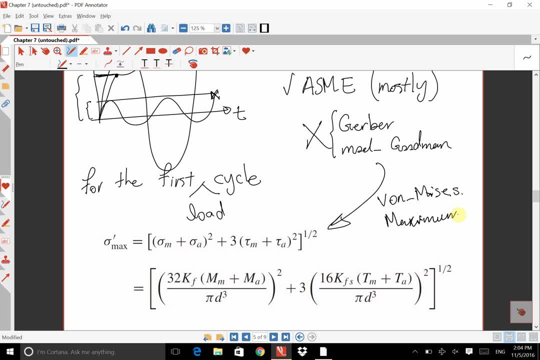 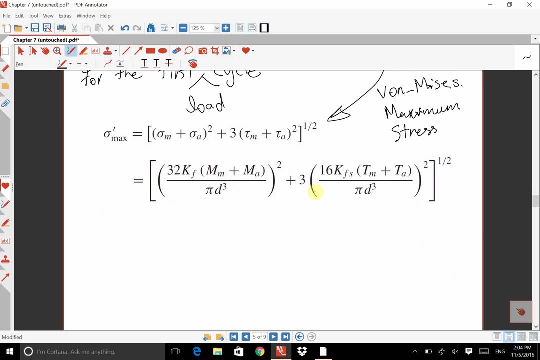 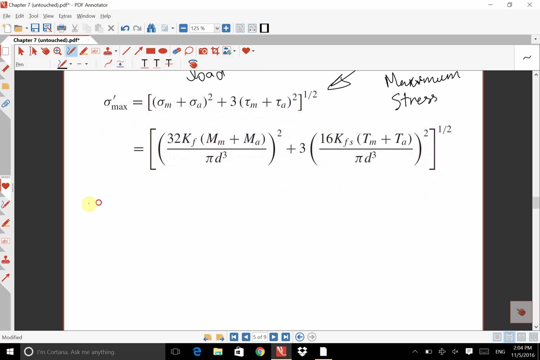 maximum stress. this is phone mysys maximum stress. so when we, when we define that stress, when you found the value of this one, we can easily check for yielding. this is what we do in chapter six and chapter four. sy divided by sigma max prime. this is what we do in chapter six and chapter four. sy divided by sigma max prime. 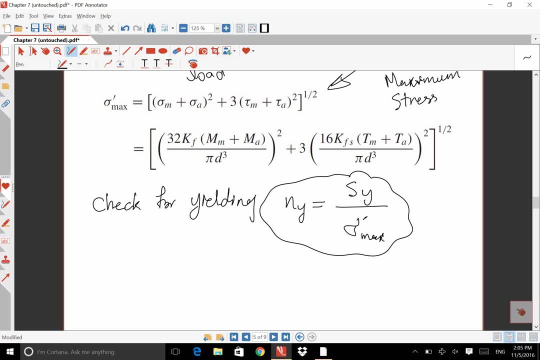 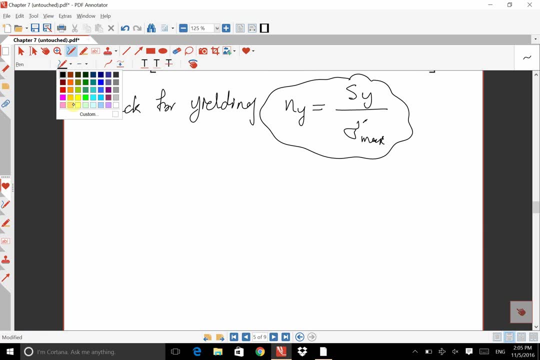 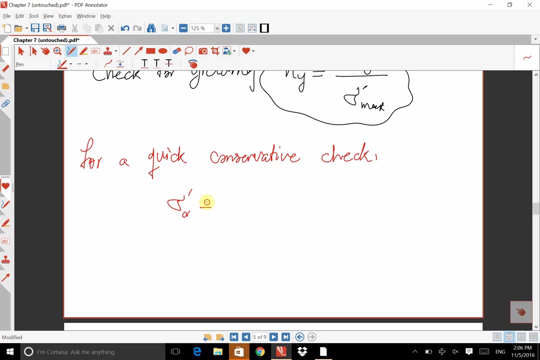 okay, that was just a checking. as for for a quick conservative way Check, we can use this method and we know that a sigma a prime plus sigma m prime is always greater than the maximum phone masses stress, and we also can use this method. maximum is equals to sigma A plus sigma M prime. That's an approximation, that's. 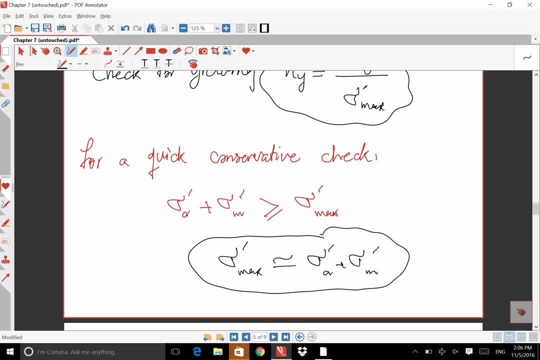 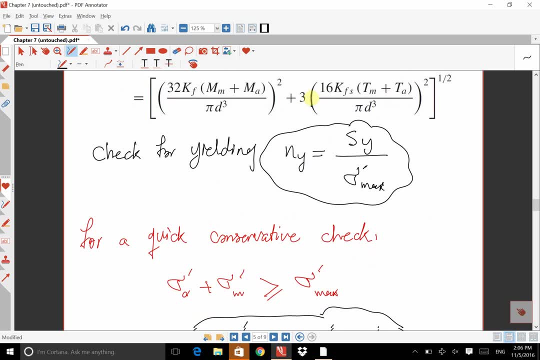 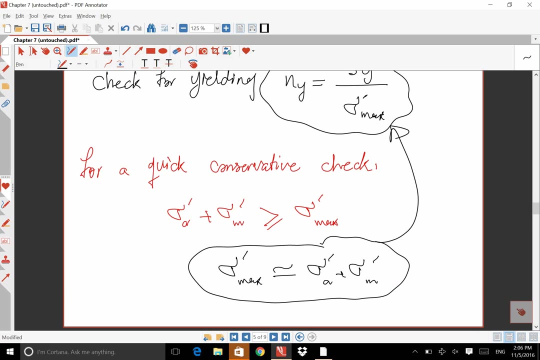 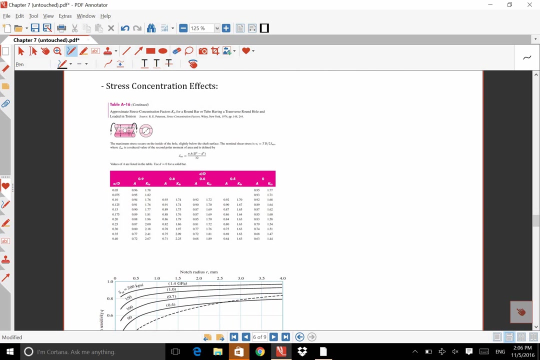 conservative because of this reason. So instead of finding sigma M prime, sigma max prime based on this long equation, we can just approximate that one with this value and then come to this equation and check for yielding. Okay, Stress concentration effects Whenever we have a shaft with some stress concentration. 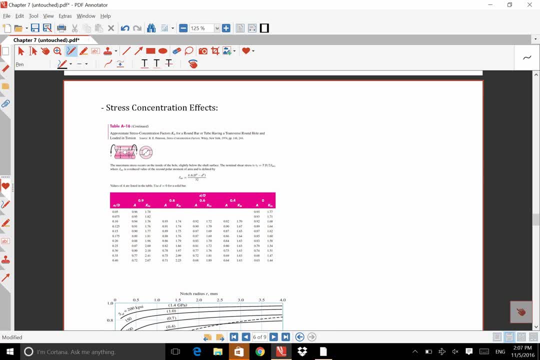 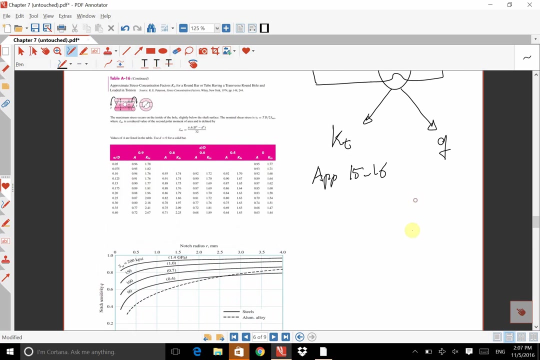 sources like, for example, if that is my shaft for this stress concentration source, here I need to find kT, theoretical stress concentration, and that's from appendix 15 and 16, and I need to find q, that's notch sensitivity. Once I get these two parameters, I can 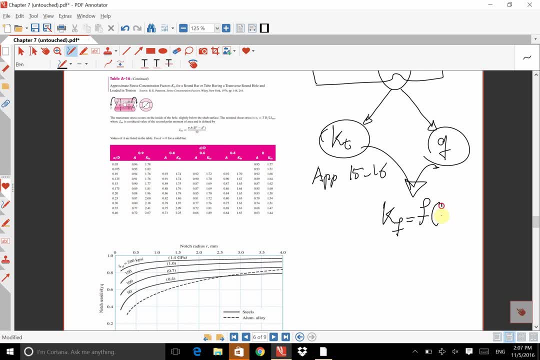 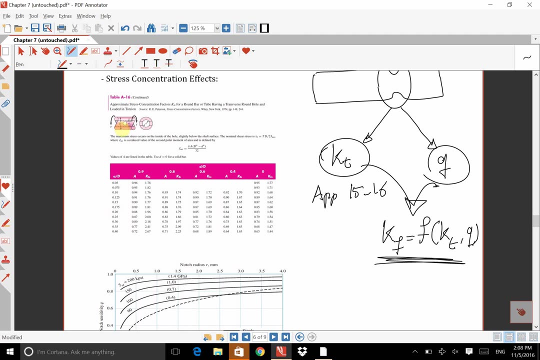 KF, which is a function of KT and Q, and this is what I'm looking for whenever I have a stress concentration, for example in this question. in this example here, we see that there is a hole in a round bar shaft or in a like in this beam or 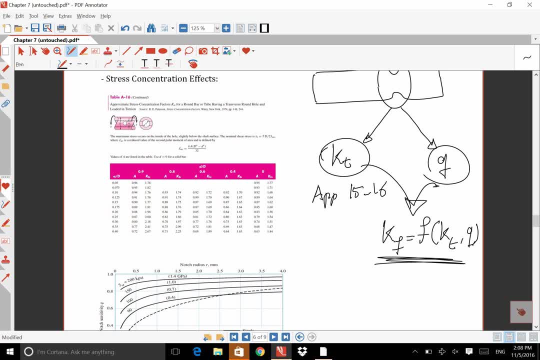 whatever it's called doesn't matter, depends on how you look at it. if you have this case with this table, we can find KT. so what you see here, this is KTS for shear, and in the table, in the previous table, in the appendix, you had KT. so this KT can be found from this table and Q's the notch sensitivity in. 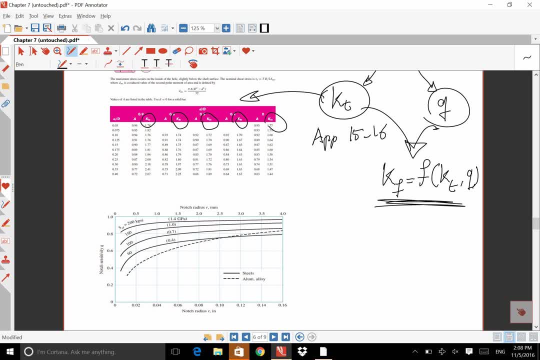 this. there are two tables for Q as well. one of them is for just Q, the other one is for shear Q, and in both cases Q is a function of R. you see, it's a function of R in metric or in imperial system, so you can find notch sensitivity for that system. so we don't 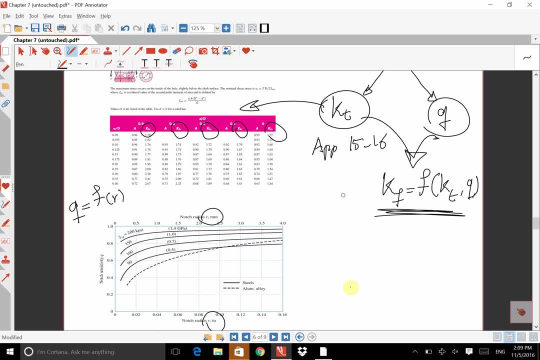 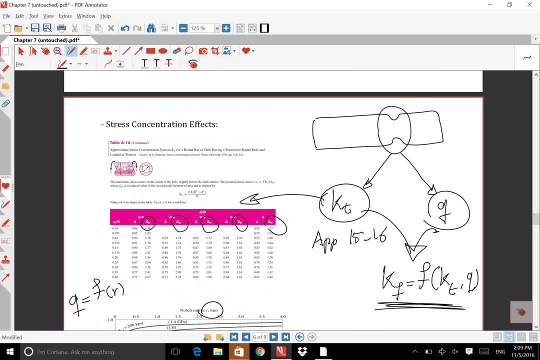 have any problem finding that Q and KT. but sometimes in some problems we might not find our stress concentration surface and therefore we're also causing this strain to like KT and it's just a matter of knowing what those are in such and such situation, but then also you also should know what that stress for. look for Q in 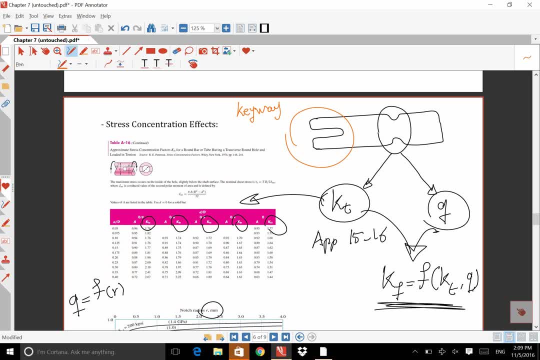 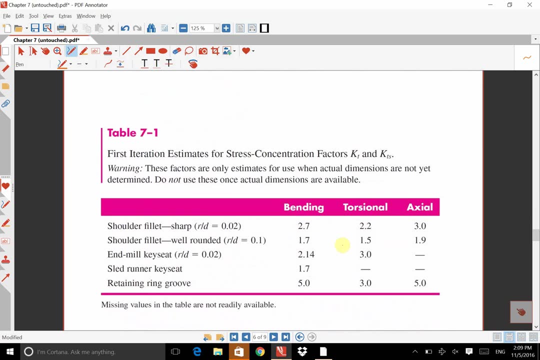 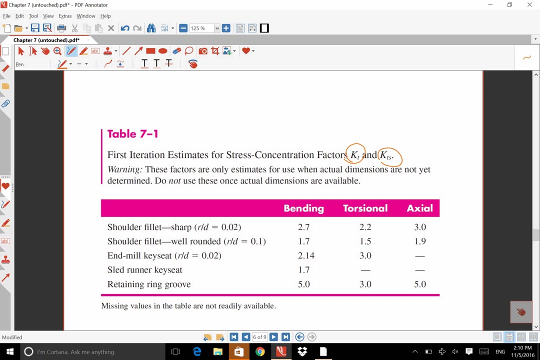 general. so let's say for the first example, if you're told that Q, T is the banget getting Vertical Aktivated, or what e is KT, in these cases we need to do some assumption. table 7-1 in Shigley's book. it gives us some value for KT and KTS when we cannot find those values in 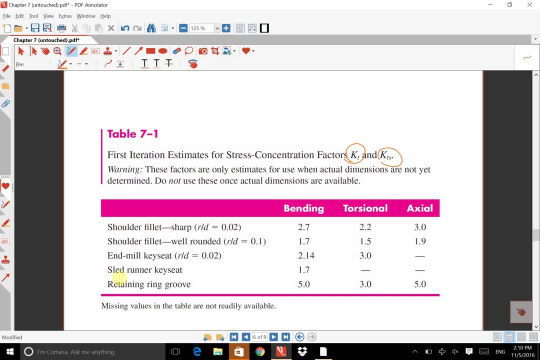 appendix. For example, in our case, if you have an end milled k-seed and if you have a bending, KT will be 2.14 and KTS will be 3, and we don't have any value here. so it means that we cannot. we don't have any information, so we cannot. 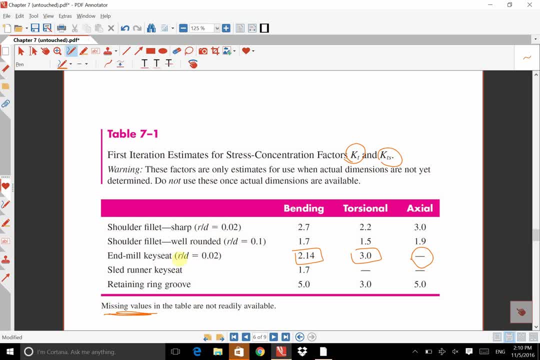 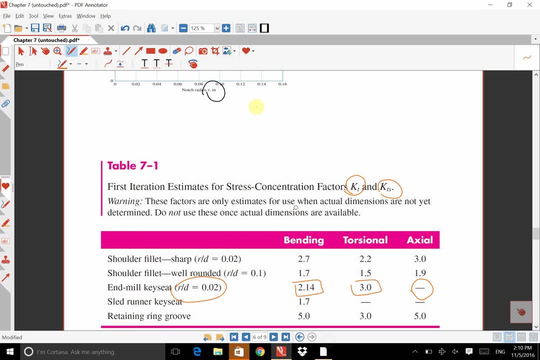 use anything at that point and you see some values here in the parenthesis, like R over D. is this much What it means? that in this case, this is the assumption that we need to use. We need to say r over d is 2% and because d is noun. 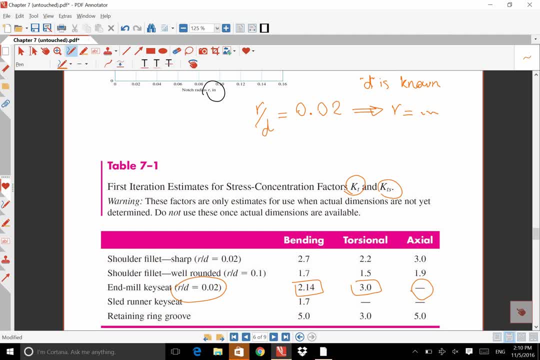 so we can find r. r is a number like 1,, 2,, 3,, 4,, 5,, 6, whatever. So once we get r, we can find q, because q was a function of r. 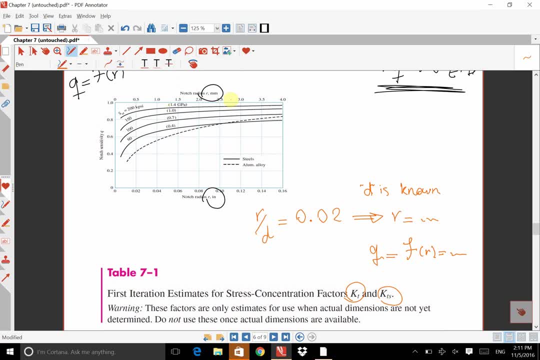 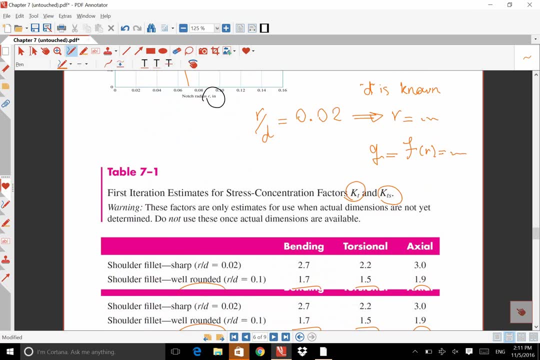 So for finding q we don't have any problem. we can just go to this table and once we know r, we can just find a line and read the r from the y-axis. So we don't have any problems for finding q. 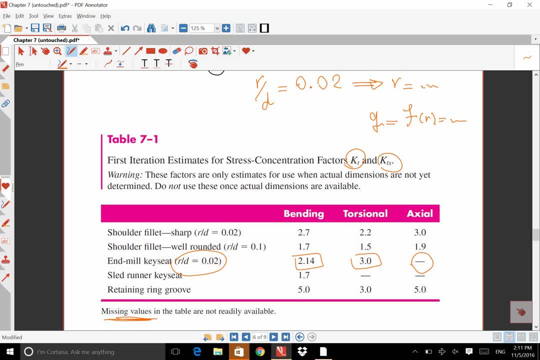 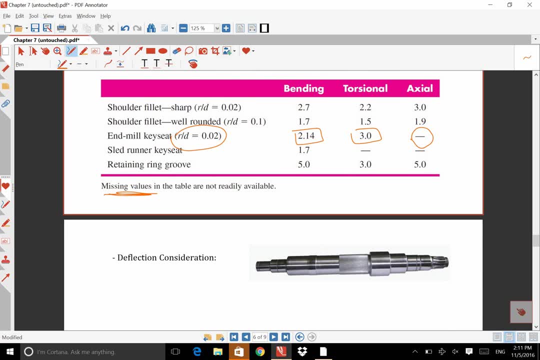 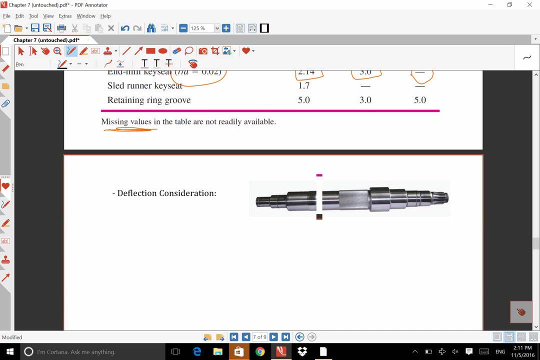 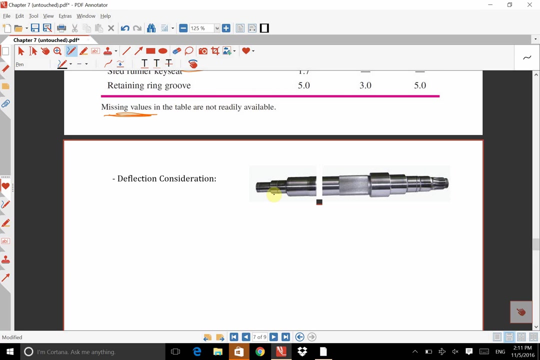 and we can use these assumptions here to finding radius when radius is not given to us. And next part, which is covered in this chapter, is about deflection, and this part was somehow covered in chapter 4 as well. Whenever we have bearing in a system, we have some reaction forces. 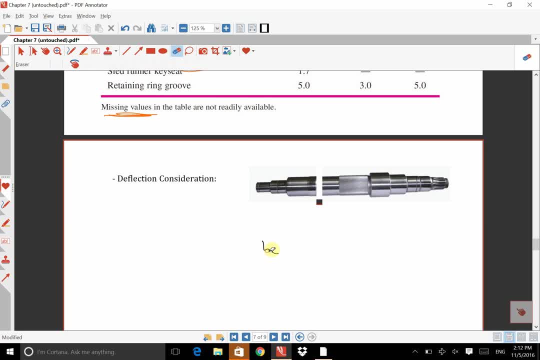 For example, if in this system, if I have a bearing at this point at point A and another bearing at this point at point B, so this means that I have a reaction force here rA and I have another reaction force here rB. 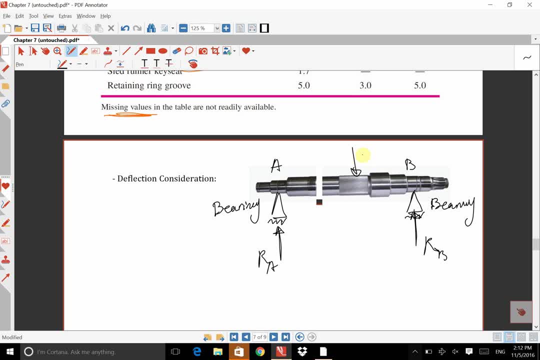 And I could have one or two or some distributed or concentrated force, let's say external force, acting on the shaft. So if I have, for example, this case after loading, this shaft will be deflected like this, and I'm going to exaggerate- 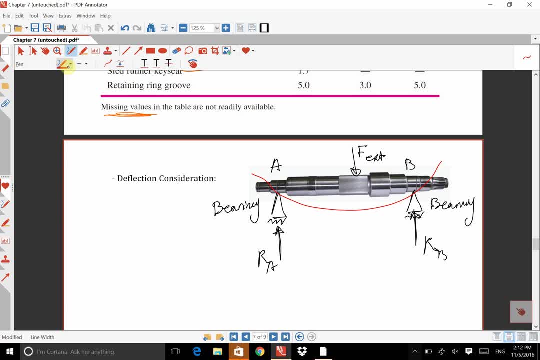 So in this part we are looking for the equation of this deflection. For example, if this, this is my x and this is my y, I'm looking for equation of y which is function of x, and this is called deflection equation. 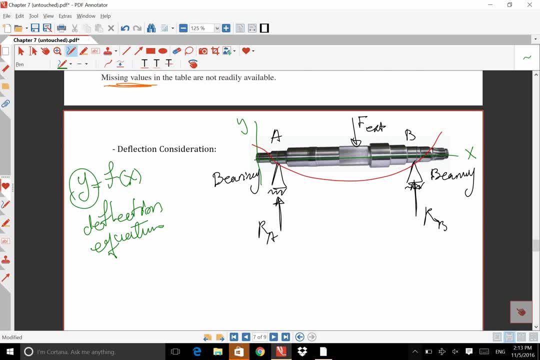 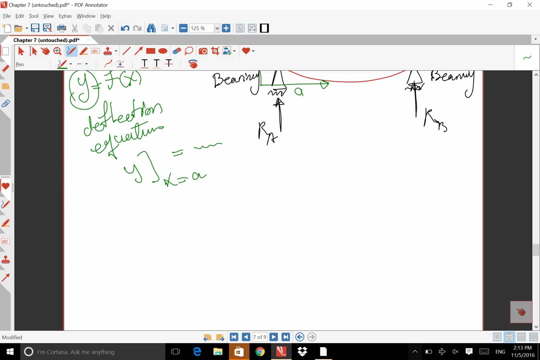 If I find this equation then, for example, if I want to find deflection at this point, I can find I can put x equals to x a and I can find the deflection based on that equation. So when we have a shaft, or when we have a beam or bar, 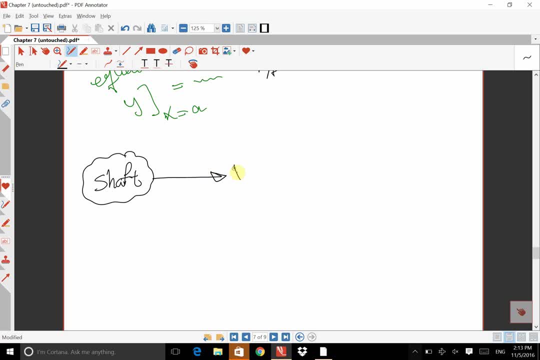 the first things we need to do, we need to find the moment equation of the system, And deflection can be found from the moment equation. In order to find the moment for a shaft, there are a couple of ways. One of them is what we learned in solids 1,. 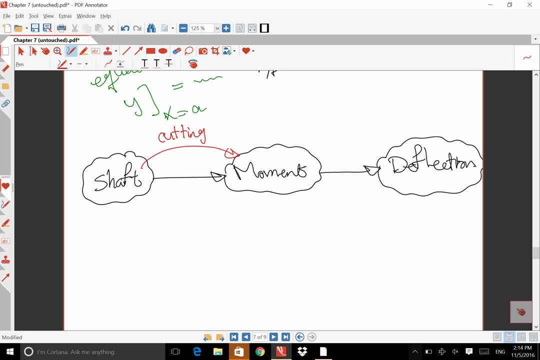 and that was cutting. when we had a shaft, we had to cut many times and wrote the v and m equations for each part, and we're going to end it up with piecewise equations for moment, The other way, which is an easier way. 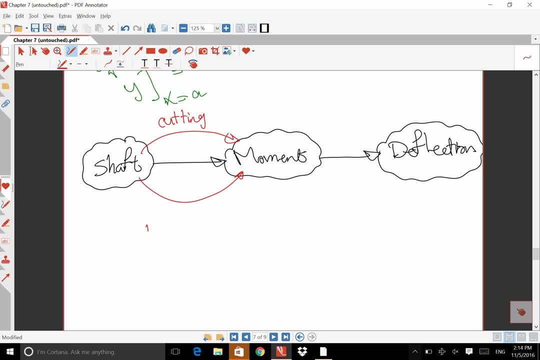 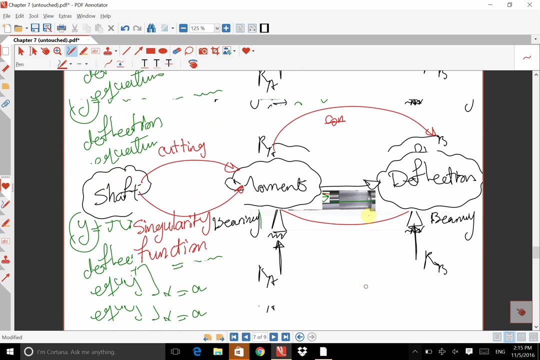 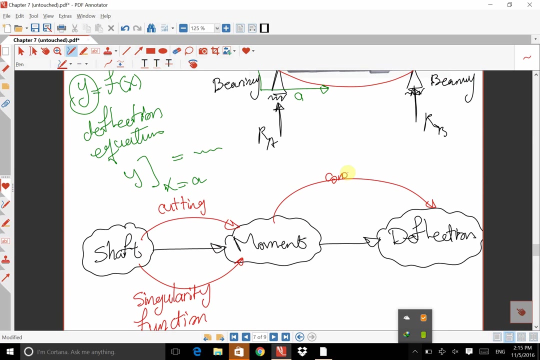 is using singularity functions Once we get the moment. now, there are a couple of ways to find deflection. One of those ways is using okay, okay. one of those ways is using conjugate methods. The other one is using area-moment method. 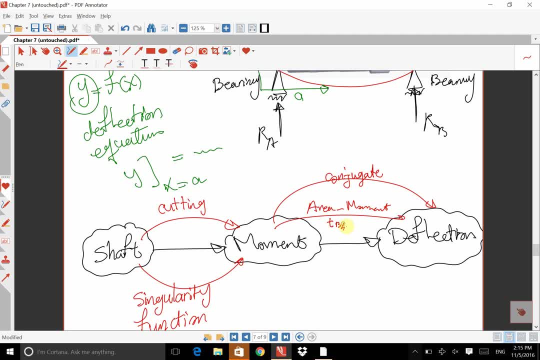 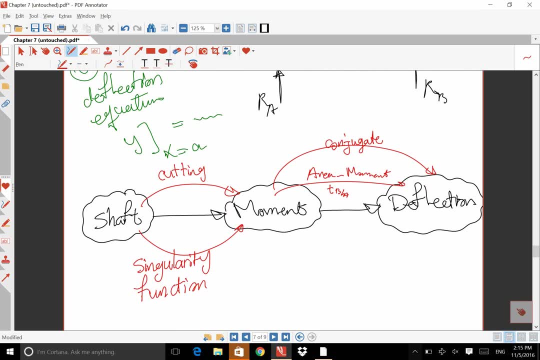 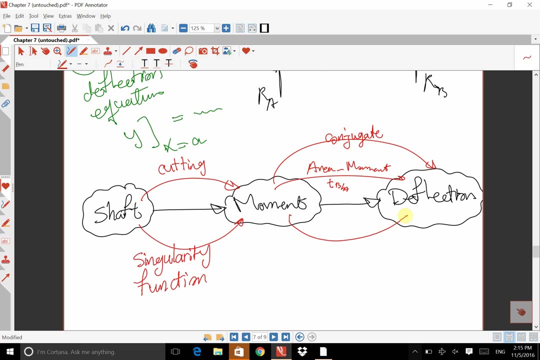 When we had something like, for example, t one point over the other point, we had to draw a tangential line and find the deflection of a point based on the other point. We learned about those things in the previous lectures, And the other way is using 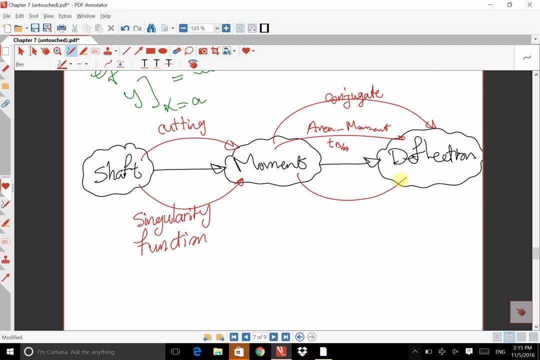 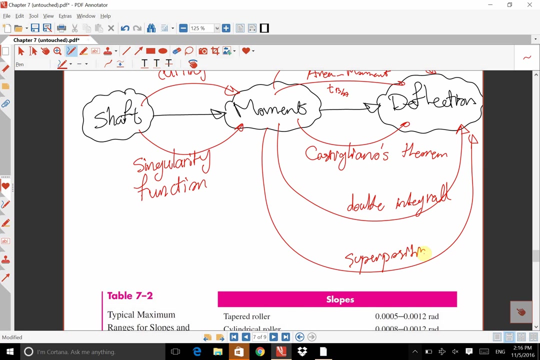 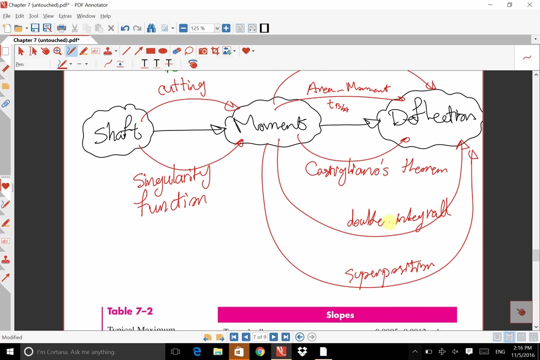 Kastick-Lnahme-Ska quotient theorem. And the other way is, when you used double integral method, we can use superposition. we learned about all these steps in the previous lectures. for example, we said that in these, you know, in double integral, in: 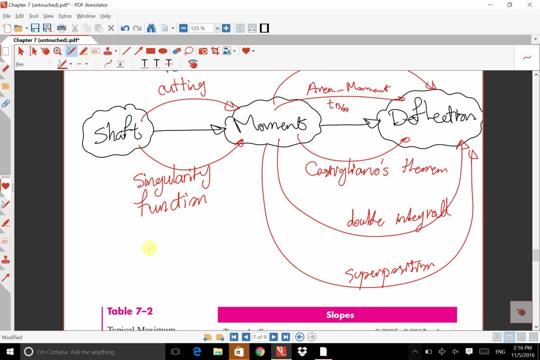 double integration method. we're gonna find Y, like we have moment at this point. okay, we're gonna find. first we're gonna find slope, which is theta by integral, by finding the value of moment over rigidity times, DX, and then we can find Y, which is integral of theta DX. this is for double integral method, for 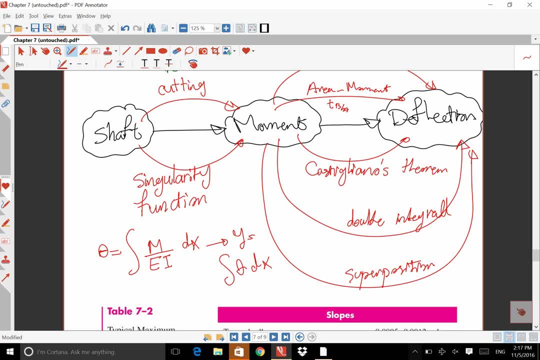 superposition. we're gonna go to a table and we're gonna find the situation, our situation- based on two or three type of cells of the, of the beam of the table, and then we're gonna add them all together and we're gonna find the deflection equations based on that. for 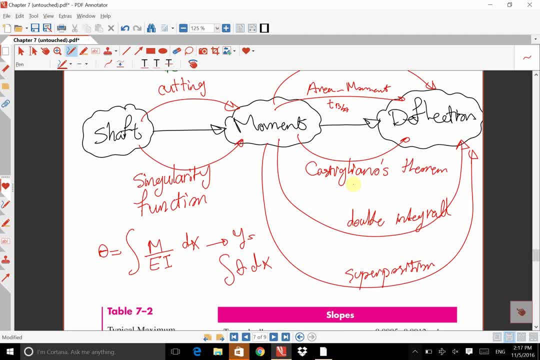 these ones you can find deflection equation. but in Castigliano's theorem we're gonna find a deflection for one point. so the difference is at this theory we don't, we cannot find the equation for the whole deflection. so this is a point. I mean, how can I say, for example, in all those in doll in doll, in? 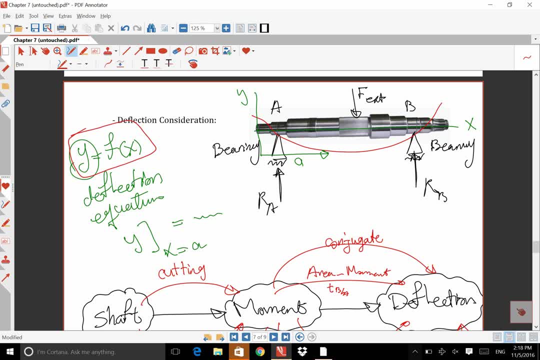 all those theories, we can't find Y based on X. so if you want to find a flushing at each point, what we need to do we need to just put the value of that point in the function and we can find the flexion. so these methods are used when we are, when we are asked to find deflections at two, three or four or more. 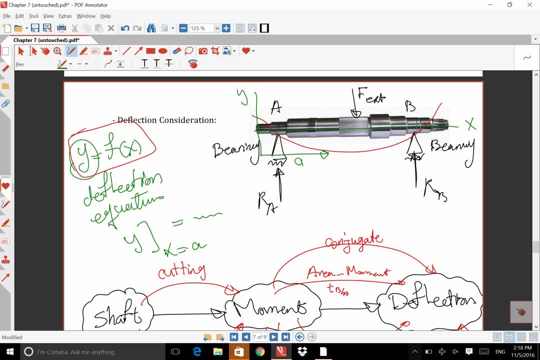 points. but if in a question we are just asked to find a deflection at one point, maybe that's easier to use castigliano's theorem, and in that theory we just put a dummy force at that point where we are asked to find deflection, at the end of the day we're going to find a number. 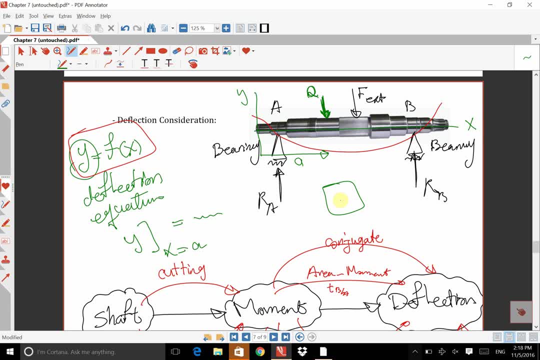 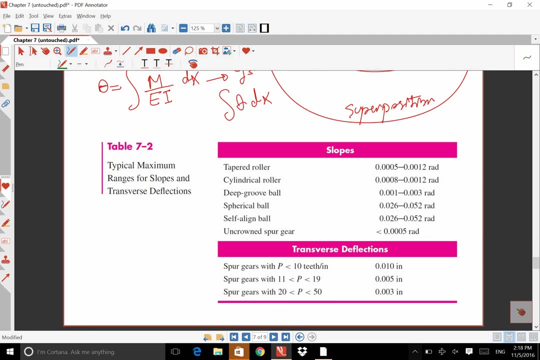 and that's number. we don't find the function, just find a number, and that number is deflection at point asked. so at point, for example, at point a, at point n, whatever, it is okay, we talk about these ones in chapter four, so we don't want to spend time in this lecture about them. 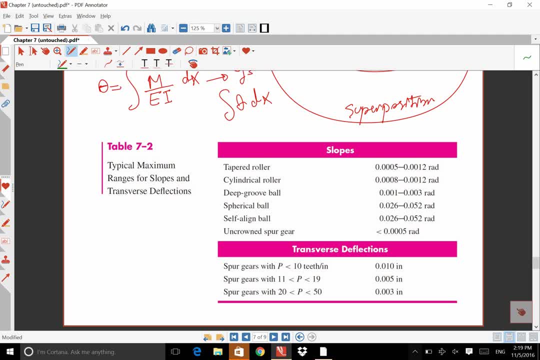 once we get those values we can just go to table 7-2 and check if we are in acceptable range or not. for example, um for deflections for spare gears with p between 11 and 19, and this much is the maximum value that we can have. so if we are less than that we are okay. if 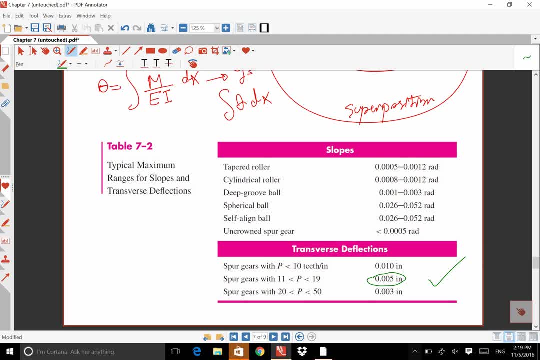 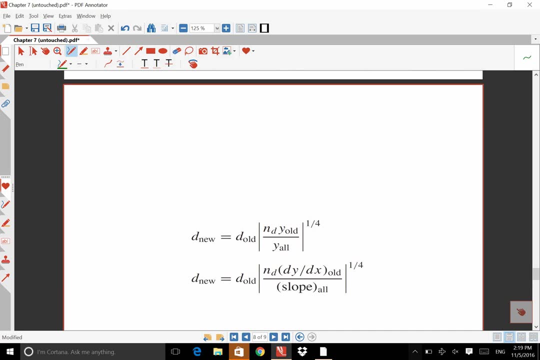 you are more. if you are more than that, we need to either change the system, change the spare gear or change some other parts of the system in order to be in a safe region again. and the first part is for the slope, okay, um, so kind of goes out a little bit with that Capital. 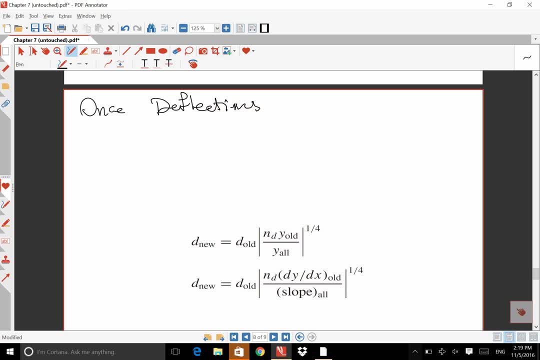 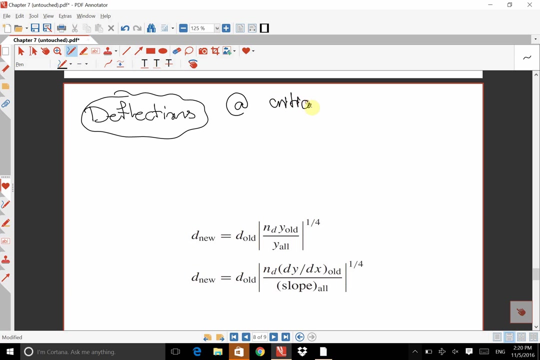 so if you come up with a very specificression, let's take a look. how can i find that? once deflections, once deflections, let me okay, once deflections at critical points. so you're always working at critical points. there are keyways, or stress concentration sources, or shoulders. 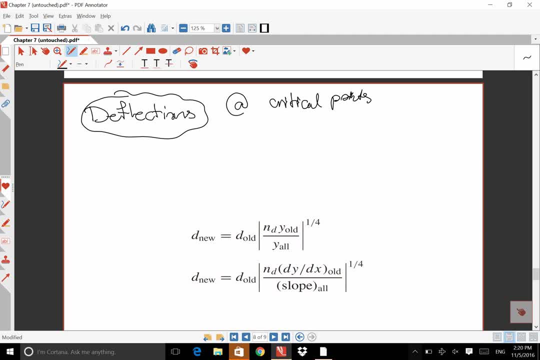 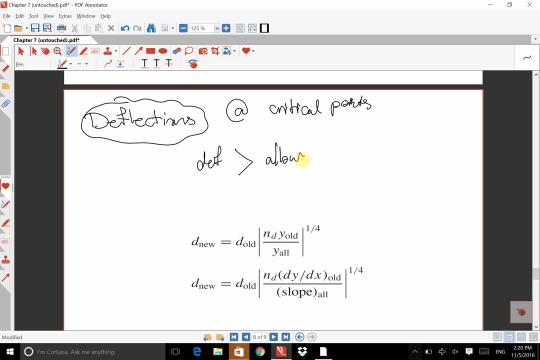 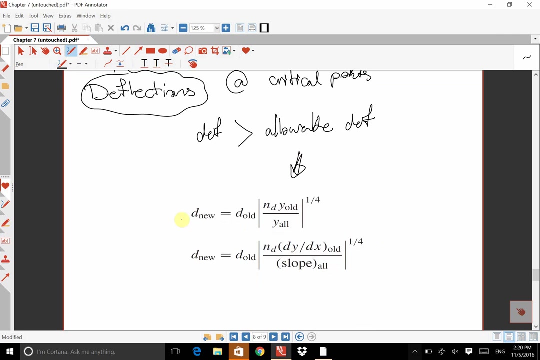 villus or these things, when deflections at these points are determined, if those deflections are greater than allowable deflection. what we need to do, we need to come to these two equations and we need to change a diameter in these equations. you see, the deflection is organizations. it is different than the other equations. 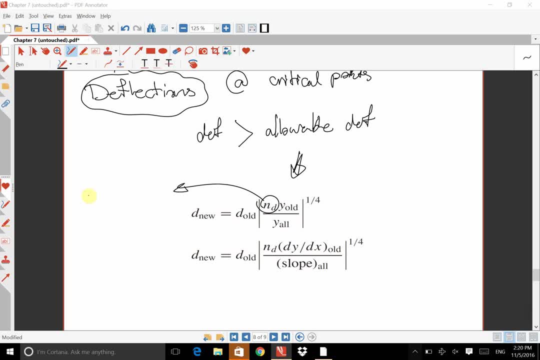 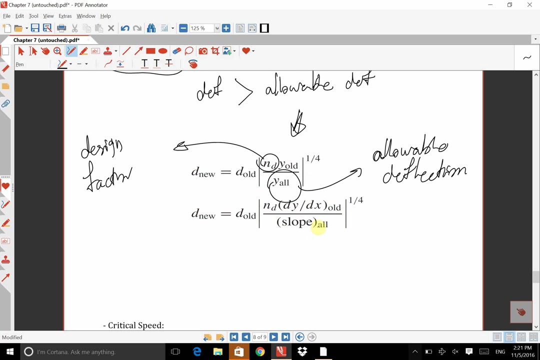 see ND. this ND is design factor. you see, YLL, that is allowable, deflection and slope I, ll, that stands for allowable. so if the amount of deflection or the amount of slope is greater than the acceptable one, we need to change the diameter, and the new diameter can be found based on these equations here. 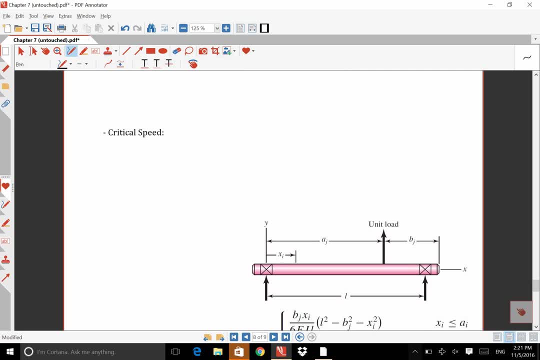 finally, the last part of this chapter which is covered in vibrations course. I'm not going to talk about this one at this point. it's about critical speed for each shaft. for each shaft, at some speed, some special speeds, shaft is unstable and that's called critical speed when shaft 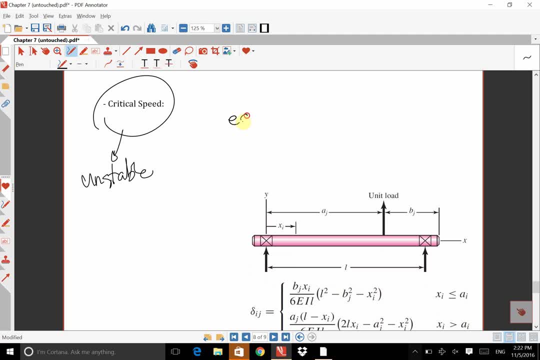 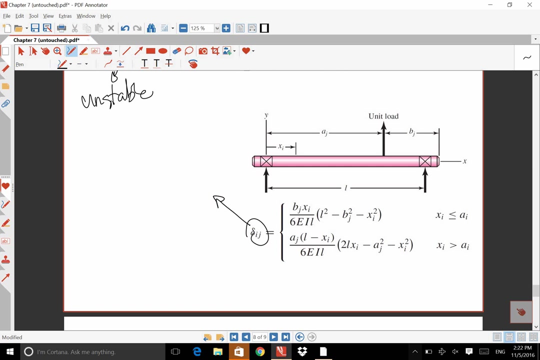 is rotating. eccentricity, eccentricity, this is C- that eccentricity causes a centrifugal force on centrifugal force, deflection, and we're going to cause, it's going to cause some problems for us, this Delta IJ that we see here. this is called influence coefficients. 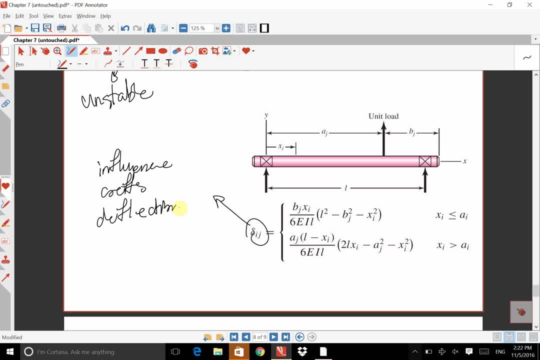 deflections at I due to a unit load- this is a unit load- at J, risen acute due to unit load at a, j. so, based on this one, this piece of the equation, we can find delta, one, two, one, three, two, one, two, two, three, three and whatever. and, as i said, i'm not 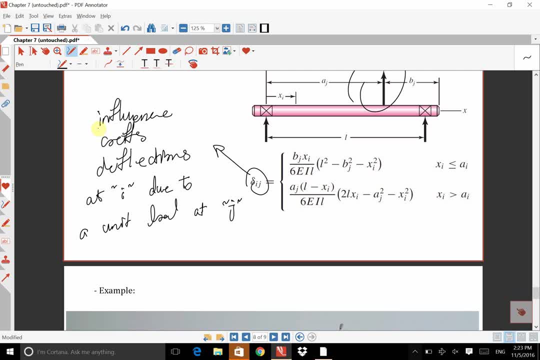 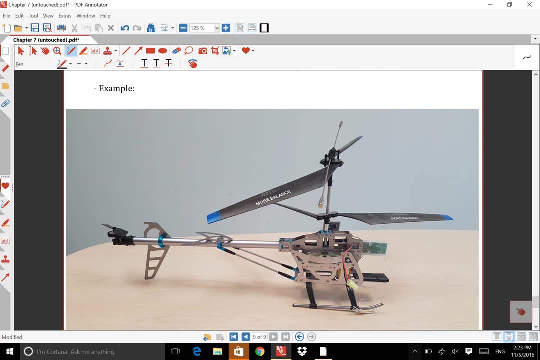 i'm not going to cover this part in this chapter. it will cover in vibrations. okay, the example that we're going to have in this chapter is the main shaft of this helicopter. we're going to study about the, this main shaft, shaft of this rc helicopter, and we're going to see, we're going to find safety factors. we're 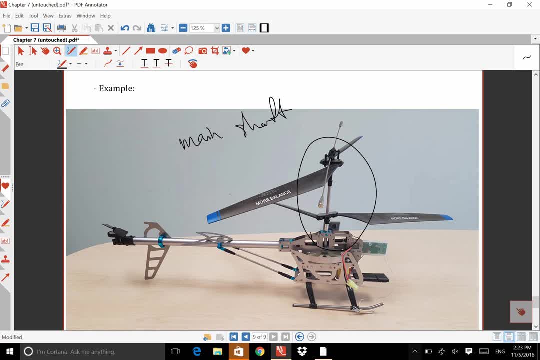 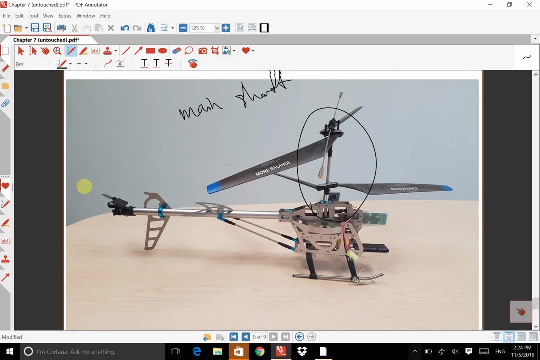 going to see all the other things that we studied in this chapter. okay, i think they're good for today and if you don't have any questions, we can finish this lecture. thank you.